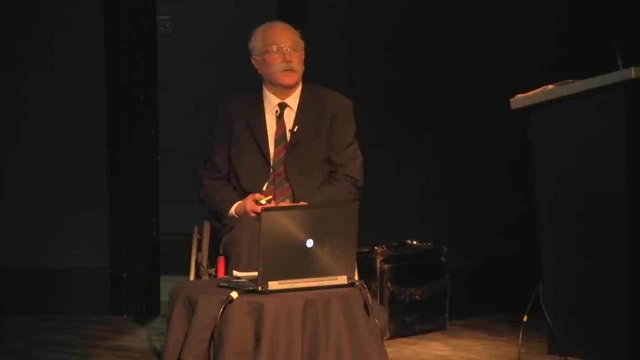 than you might imagine, I started my PhD in 1960. And at that time I was interested in trying to see how one could use Roman and Greek and Phoenician classical ports to measure the sea level change around the Mediterranean. I constructed an inventory, by the time I'd finished, of about 1,100 classical 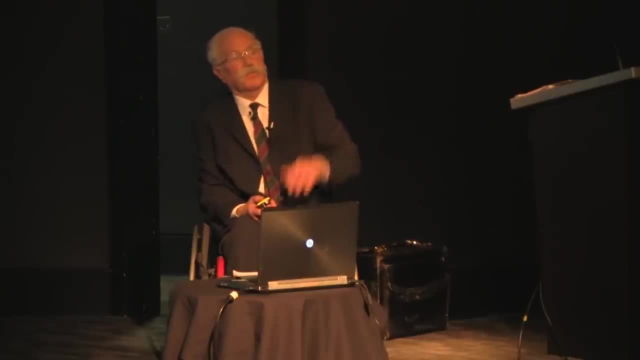 cities And they're not all underwater. But obviously if a city is built on the waterline, with docks and jetties and breakwaters, it's going to be a very, very difficult thing to do. But if you're building on the waterline with docks and jetties and breakwaters and so on, 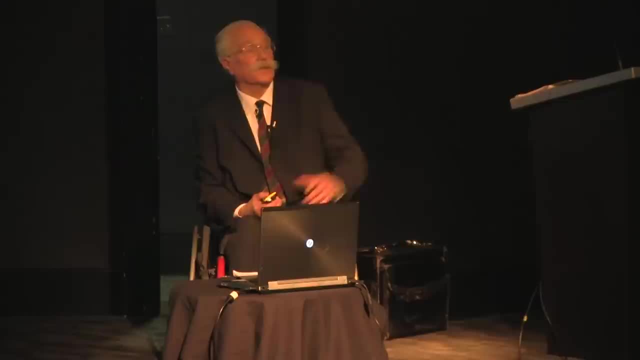 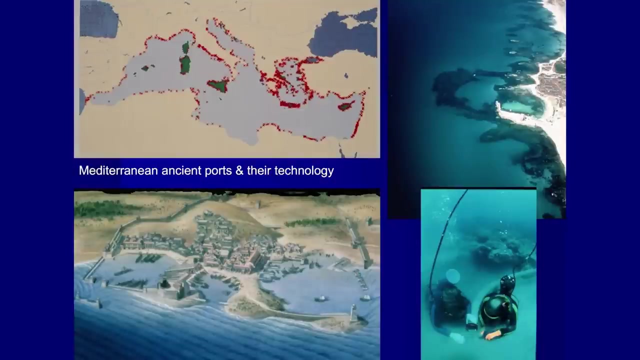 the footings of many structures are in the sea, So that from this and from the building, such as mosaics or temples or roads, which had to be on dry land, you could work out the change of sea level. Examples that: Caesarea, on the coast of Israel, And this is the Crusader Fort, But that's. 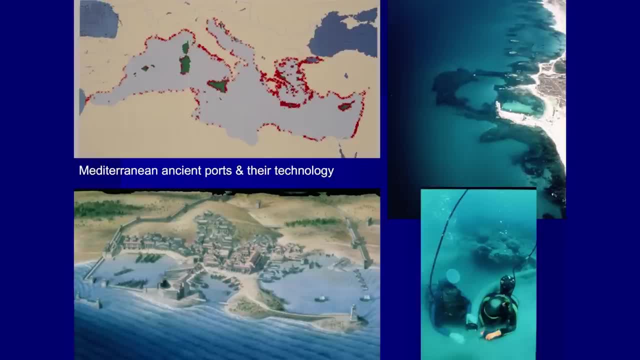 the ancient breakwater built by Herod, with all sorts of concrete structures and jetties. there These are divers in Israel working on the remains of Caesarea, And this is a reconstruction of a typical classical port. I made a little sketch drawing for it And a commercial artist. 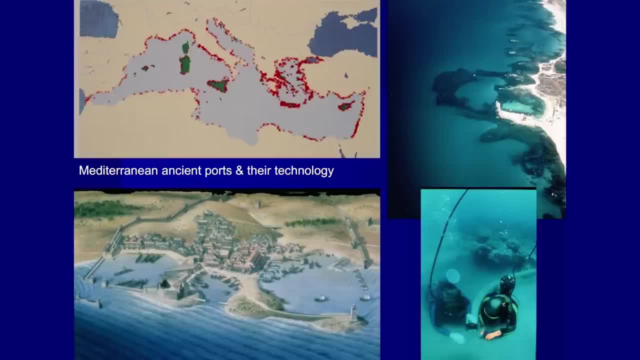 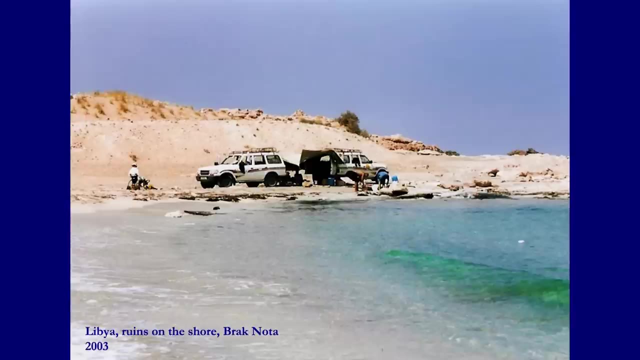 put together this very nice visualization where you've got the military port here with slipways and triremes and so on, and fortified entrance, a fishing port which is much smaller and a big commercial harbor for grain vessels and so on. This is the life I love, Libya, 2003.. And we've got the ruins of Braknota in the sand. 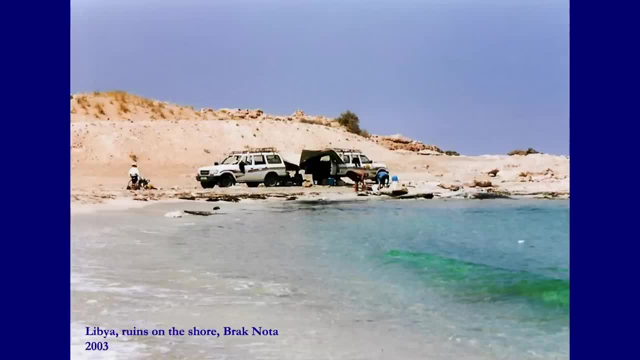 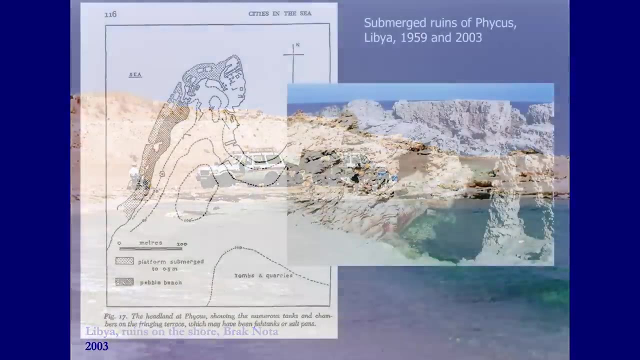 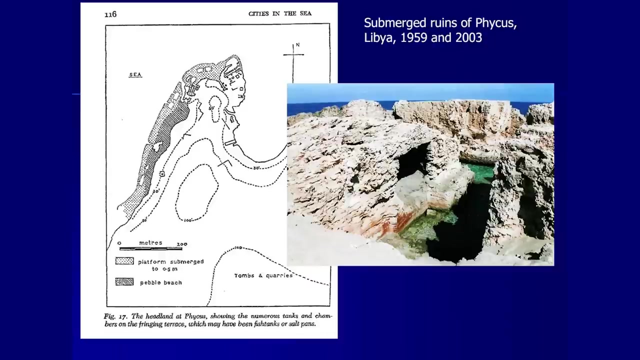 Two desert-converted Toyota Land Cruisers. Our children, Peter and Kirsten, are in there somewhere, and Jay And the drivers getting ready to make a fire for lunch and me working on the notes. It's hard work, OK, Ficus. This is on the coast of Libya. It's a site which I first visited in 1959. 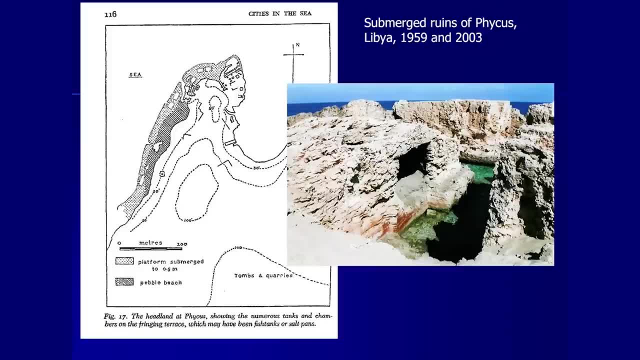 and made this map which, as far as I know, is still the only reasonably accurate map published of it. You can see these extraordinary structures: rock cuttings, huge incisions in solid rock, leaving things rather like roads with rooms and, in this case, a little. 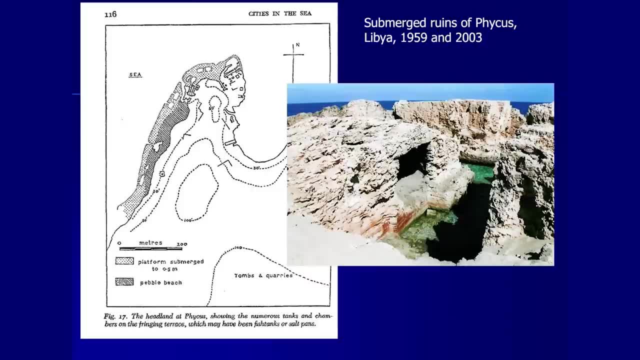 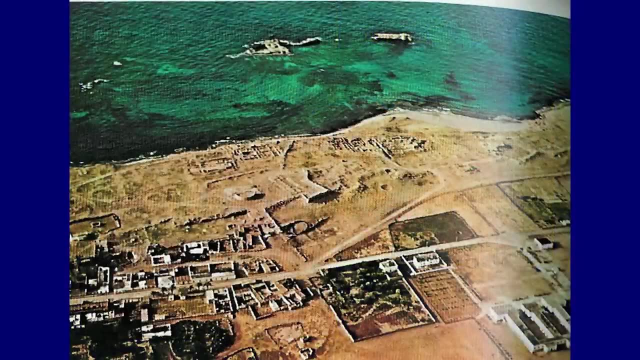 sort of temple with an offering inside A little niche And nobody really has a clue what it was for. The channels here are flooded. It's probably submerged by about two meters. Along the shore we have Apollonia, which I first visited in 1958.. This photograph was 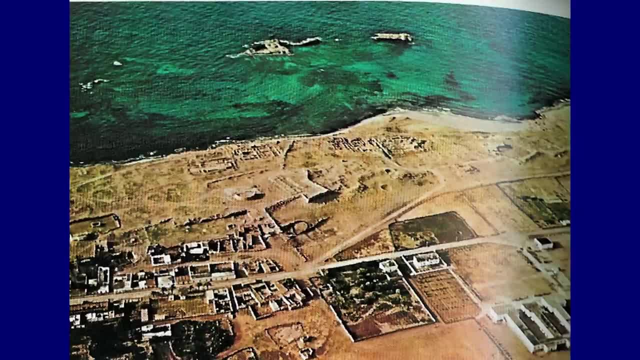 taken in 1957 from a military helicopter, And this whole area is the flooded town. And that's the outer harbor, That's the lighthouse And these are the slipways. OK, So this is the outer harbor, That's the lighthouse And these are the slipways. 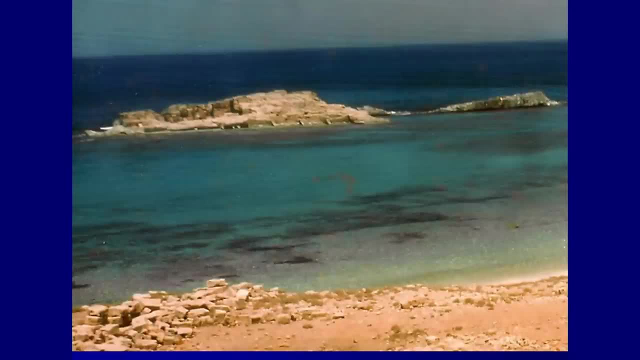 This photograph was taken through polarizing sunglasses to cut out the glitter in the water. The perspective is rather misleading Because of the angle. it makes it look as if the island's very close to the shore, But that's about 500 or 600 meters You can see. 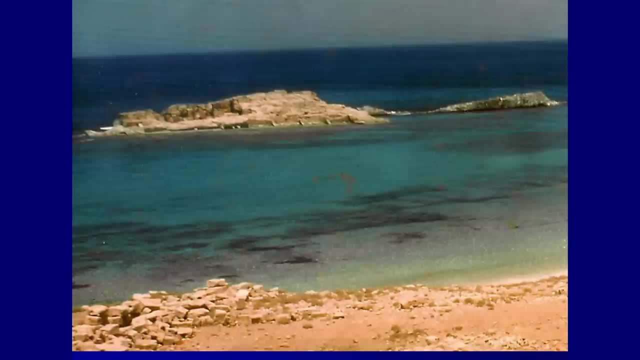 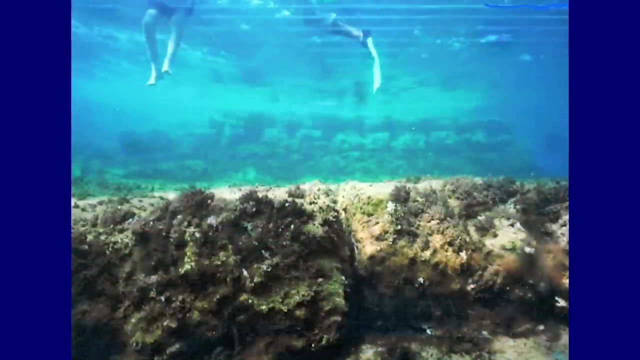 the tops of the slipways along here. There's a row of buildings here which we call the Nine Keys And the sandy floor of the harbor basin. And the sandy floor of the harbor basin is in there. Those are Kirsten's fins on the right and my feet on the left. I don't wear fins And 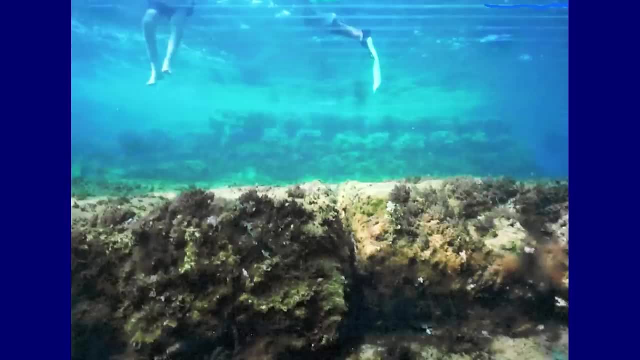 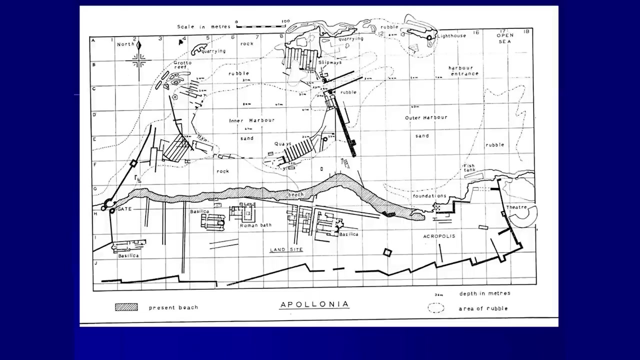 you can see the foundations of a huge fortress tower there, And this is the one on the other side of the channel guarding the entrance to the harbor. This was the map which I made with a team of eight divers from Cambridge in 1958, and 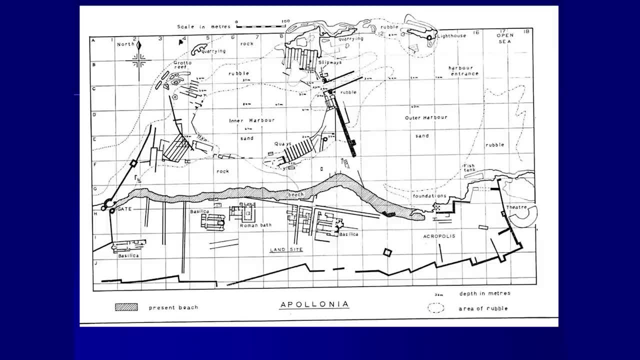 59. Try and imagine this is before plastic, before plastic tape measures, before GPS, before laser range finders and before a lot of other things. We were given a box of plastic bags by ICI to see if we could find something useful to do with them. 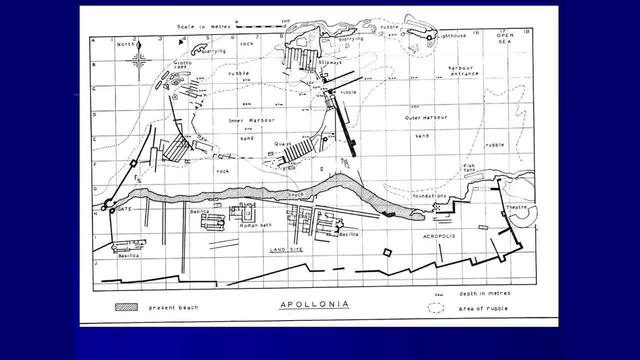 They were very useful. This was all done by a very simple theodolite, and station pointer Nick Wood did all the hard work on this. This is a map from the design of the survey system. This map has never been superseded. 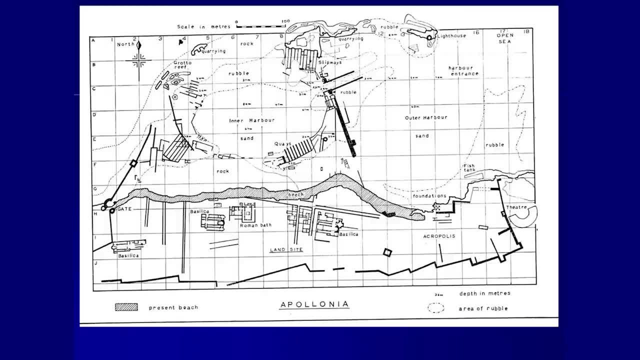 much to my annoyance. I mean, it's absolutely disgraceful that 50 years later, the maps are getting worse and worse. I sometimes feel like a sort of medieval monk who comes back a thousand years later and find that beautifully illustrated manuscripts have been degraded. 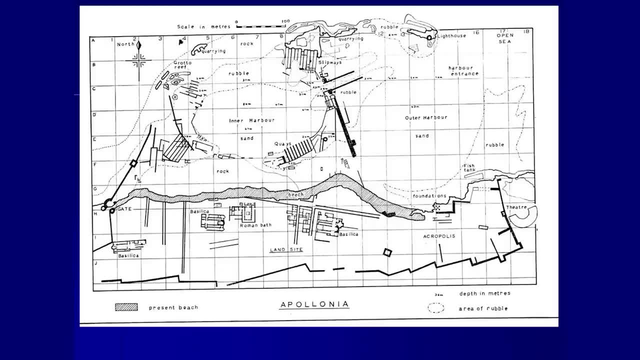 by photocopying until there's almost nothing left. If you look on Wikipedia, you'll see I had to put this map on Wikipedia Because the map that was on there before showed almost nothing, And people keep trying to simplify this and sort of summarise it in a way which is completely incorrect. 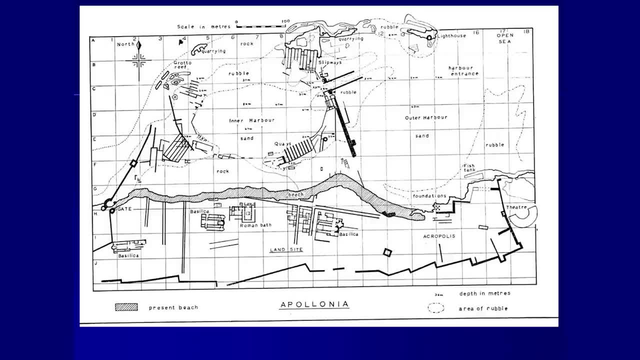 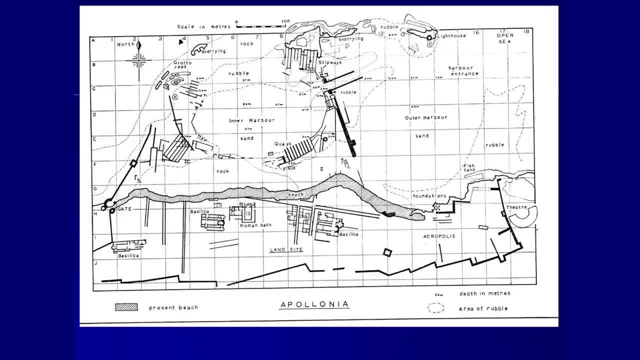 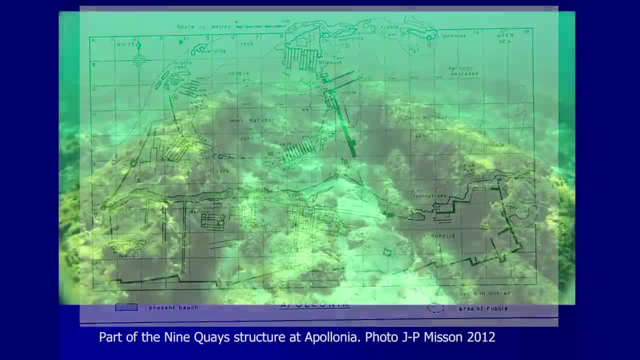 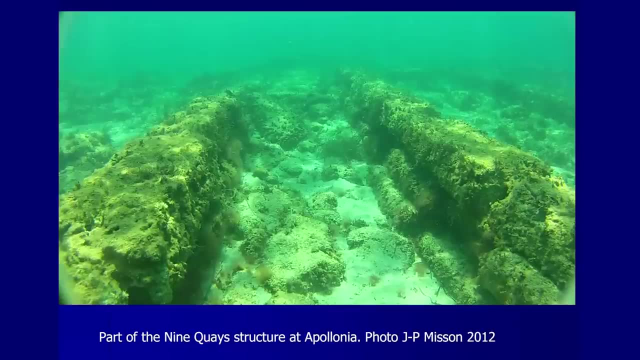 building this area had tunnels through the reef with a roof still in place. I've got that on movie. this is a photograph of the nine keys by Jean-Pierre Misson, who was born in Libya and swam as a child here almost every weekend and keeps sending me more and more photographs. he's a 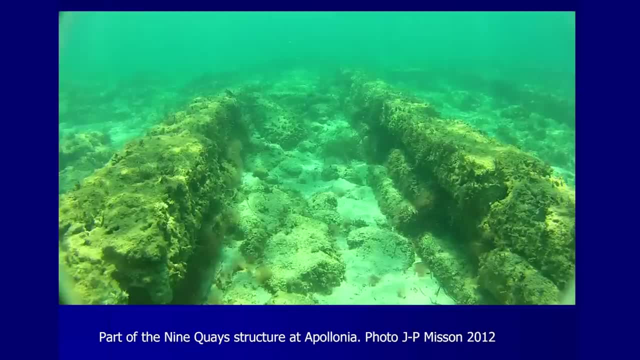 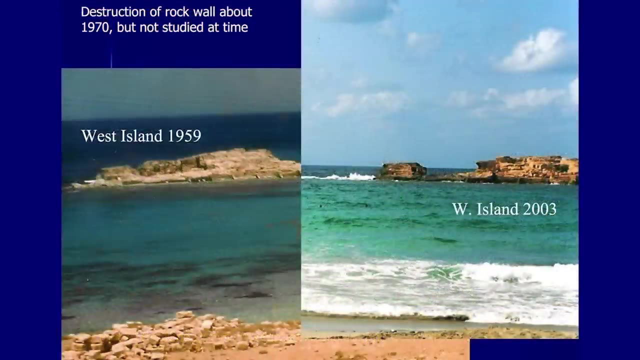 remarkable source of information and you can see the masonry structure and at the end there, the whole of this area was filled in with blocks to make a key and there are nine of these with gaps in between them, and the ships would have come in between them in 1959. the island, West Island. 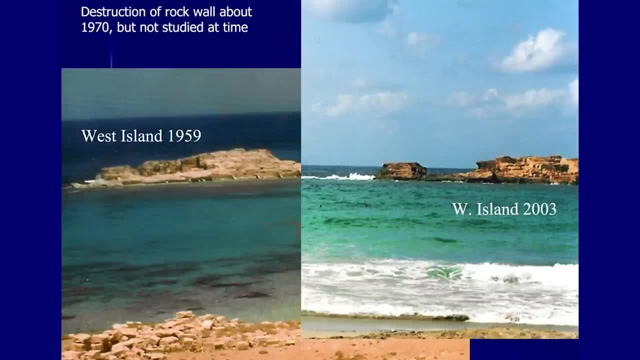 was continuous. this was a work area for servicing the ships that came up on the slipways. this area is hollowed out. there are caves and so on. inside, every inch of this island is a carved technological creation. in 2000 and 2003 it looked like that that wall had gone. 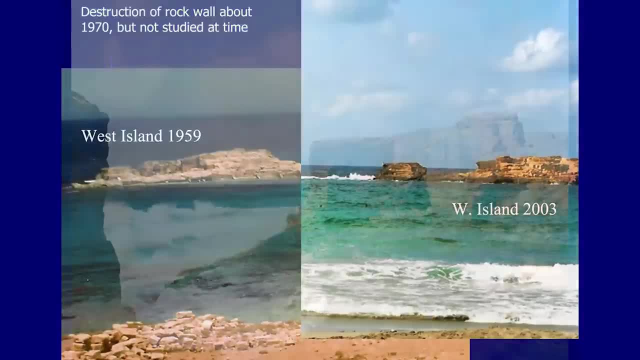 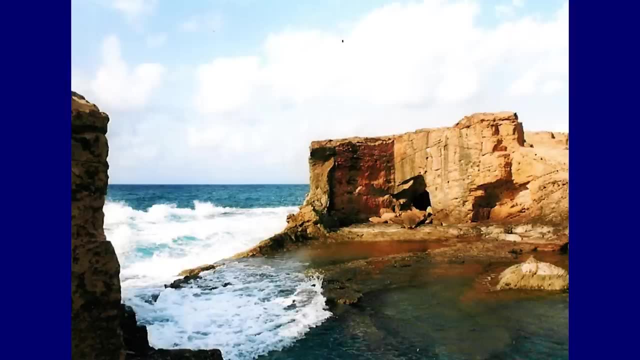 Jay Kleinberg took this photograph and you can see there's a gap about 20 meters, two meters thick and about five meters high. look, there's the wave trap outside and the waves are now breaking across the island and washing sand onto the center of the island. Jean-Pierre sent. 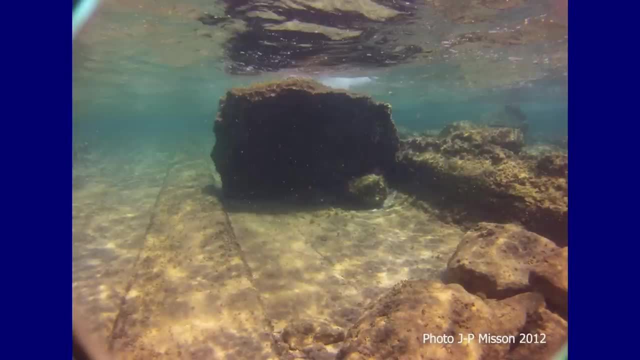 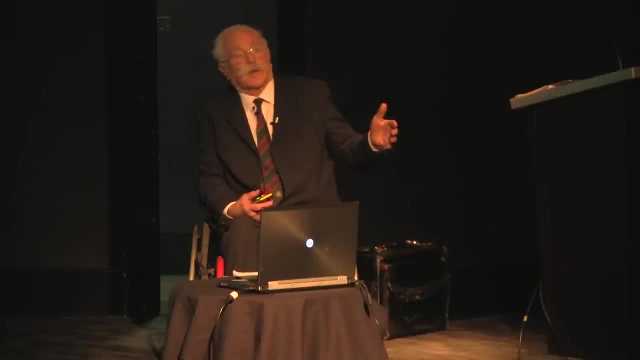 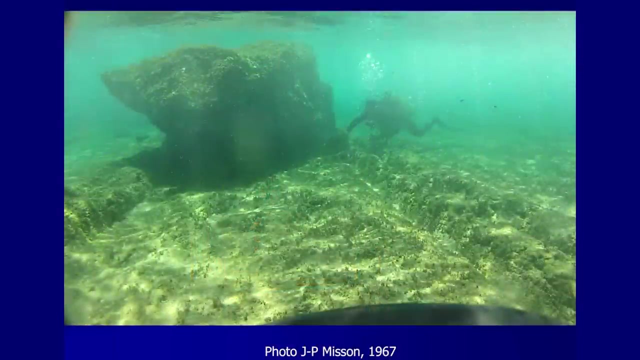 this happened when we were there in 2003. we discussed with the French archaeologists, Monsieur Laronde and his staff. when that wall broke, nobody knew. the villagers in Massachusetts didn't know. but through correspondence with Jean-Pierre Misson, he sent me this photograph yesterday, which he says was taken in 1967. there's another block. 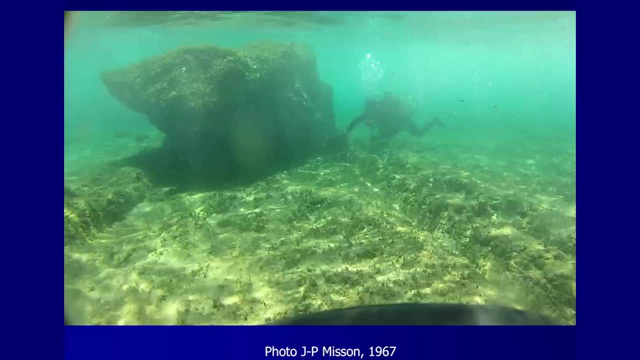 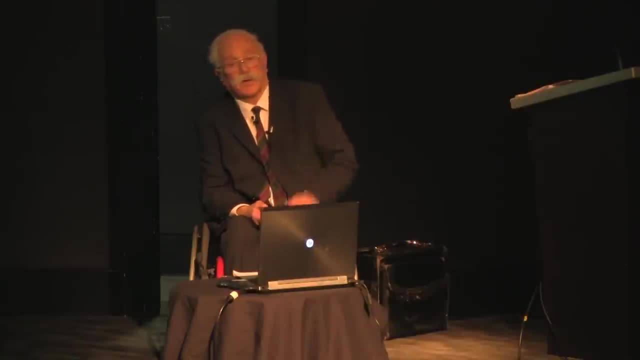 lying on the slipway and a diver and that means that the that broken wall at the back was smashed through somewhere between 19 in the early 60s, somewhere between 1959 and 67.. there are certainly tunnels on Grotto Reef and other things carved through the solid rock which have also been smashed. 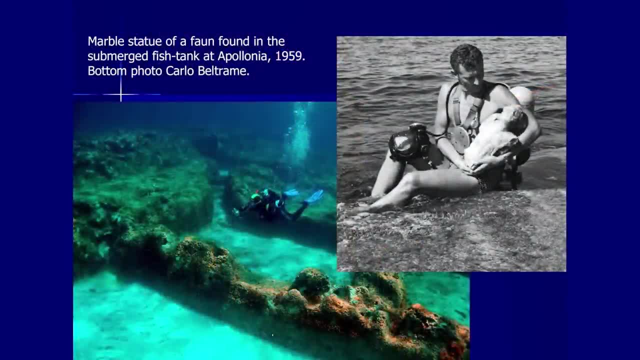 the fish tanks here. piscina- this is a piscina loculata, which means that it had rectangular tanks that are divided. it's about 50 meters by 15.. that's the walkway where people would have gone around the fish tank to be able to feed the fish and see that everything's all right and channels. 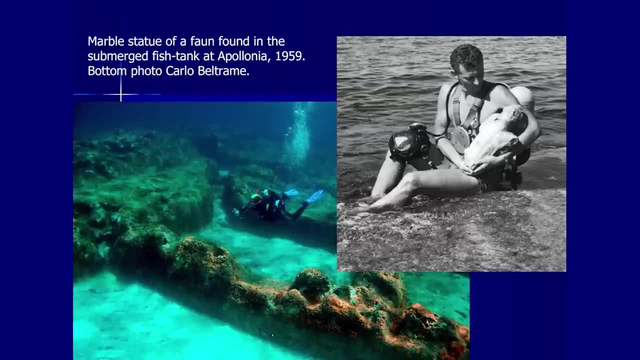 with sluice gates to control the flow, which is tidally controlled because the there is a tide of about 10 or 20 centimeters in the Mediterranean and by opening and closing the gates you can get the water to flush and keep the tank fresh. we found this small marble fawn in the tank in the 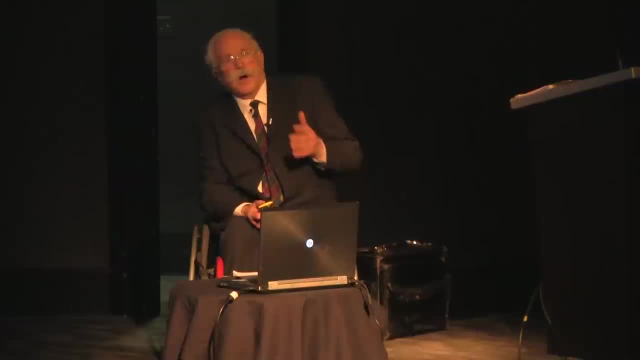 tank in 1959.. okay, up to this point I've been talking about classical sites. what Michael ordinary underwater cities back to 2 500, 3 000 years ago. as we go further back in time that things start to get more interesting. if a site is unconsolidated, it's not square blocks fitted. 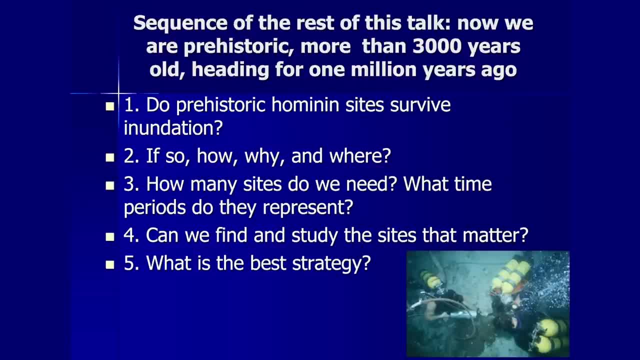 together- ash law, things held together with keys and dovetails and so on, but just uh. and then, um, earth and bones and flints- will it survive the sea level coming over it? if so, how, where and when? when i say, how many sites do we need? finding one site is just a sort of gimmick. um, it's a thing. 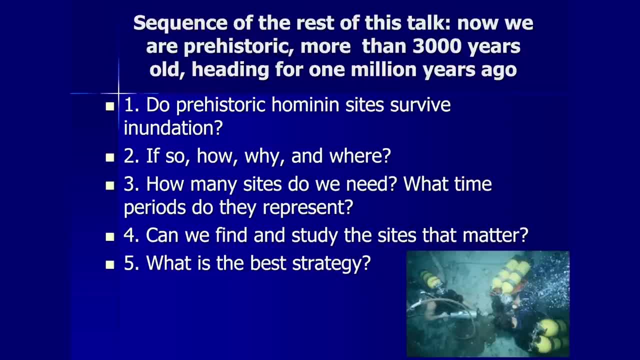 you can't work out very much about a population, about habits, about variability, about hunting or diet or whatever, from one site. you need to study a geographical area and find a typical site spread perhaps over hundreds of kilometers. can we find and study the sites that matter and what's the best strategy for doing this? okay, we're now starting to move backwards very rapidly. 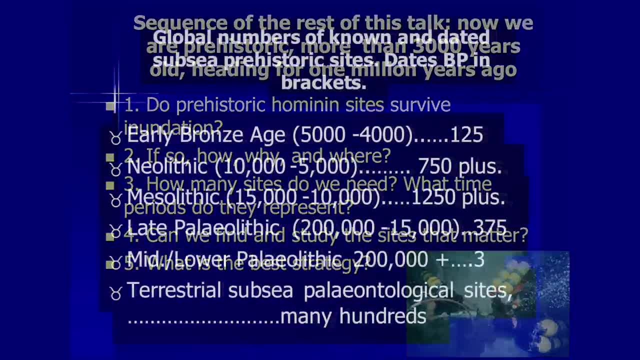 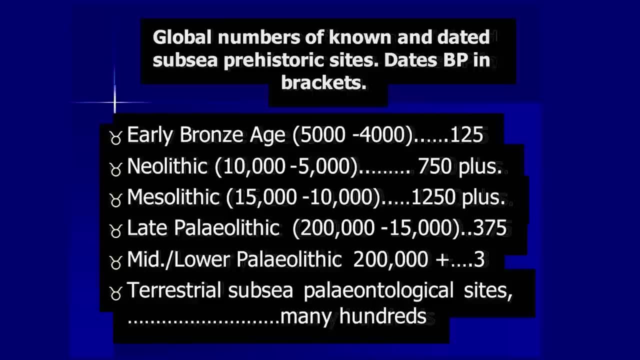 just to give you. this is not a detective story in which i keep the solution to the end. i'm giving the answers as i go along. how many bronze age sites do we have in europe? this is a data set from european projects about 125 sites underwater. 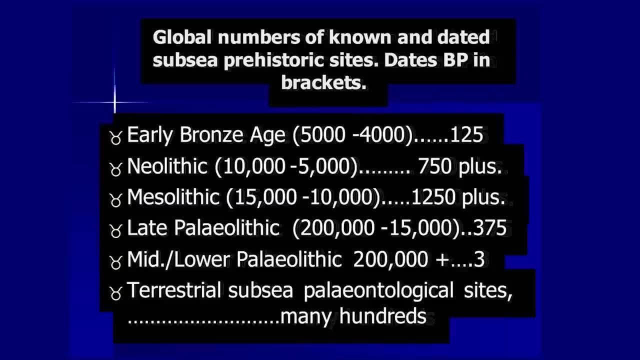 neolithic, that's in the date range five thousand ten thousand years ago, 750 prehistoric sites underwater, mesolithic, 1250. okay, so we're not dealing with just one or two finds. prehistoric sites have survived under the sea in european waters in their thousands. late paleolithic- this. 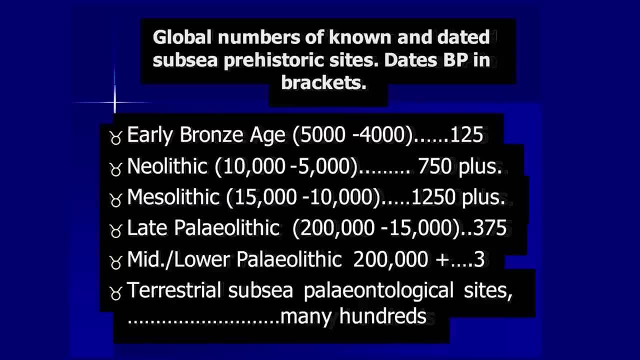 one surprised me when we went through the database which we've built up in the last few years. we've already got 375 sites older than 15 000 years underwater and there are many hundreds, if not thousands, of sites where people are finding the bones of mammoths and woolly rhinoceros and that sort of thing. 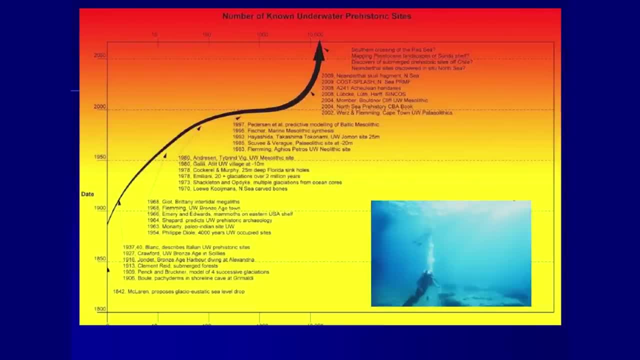 this is to show again that the subject has been studied for many years. the number of sites that we i think they've is the number readable there. the number of sites here goes up to about 10 000. this is the date starting in the 1800s. 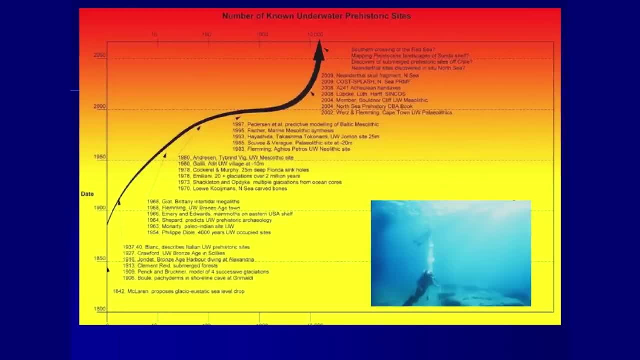 and coming up to the present and when the scope of the ice ages was first realized, around 1840, mclaren very quickly calculated that if you put so many thousand cubic kilometers of ice on the land, then the sea level will drop by tens, if not hundreds, of meters. 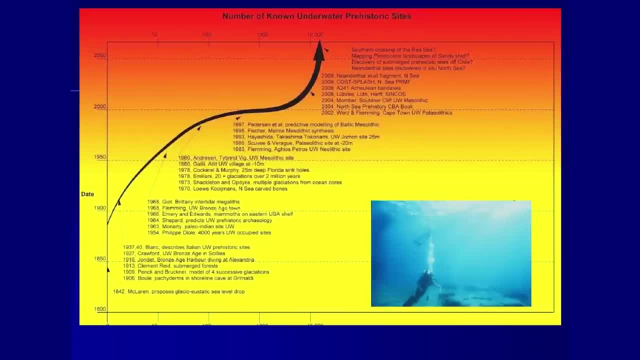 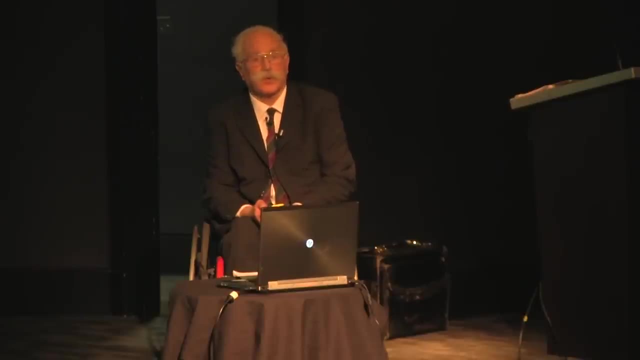 and a few years after that people realized that mammoths and tigers and vegetation and rivers and so on would move out onto the continental shelf, and people probably as well. that's the way it is now. fishermen occasionally pulled up flint tools or even human bones which look very old fossils. 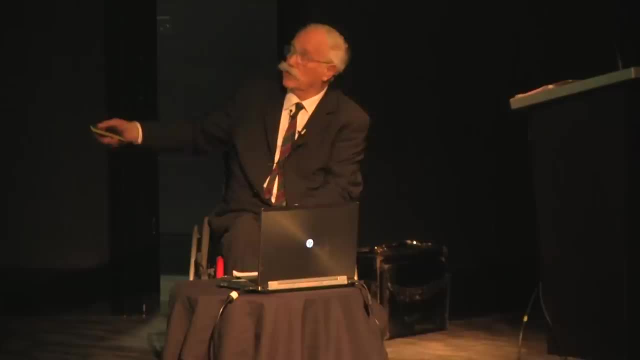 and people realized quite early on- by 1900, 1920- were publishing papers showing that there was evidence for human occupation of the continental shelf. when we get up into the 50s and 60s the number of papers begins to accelerate, and now, through what we call the splash cost project, 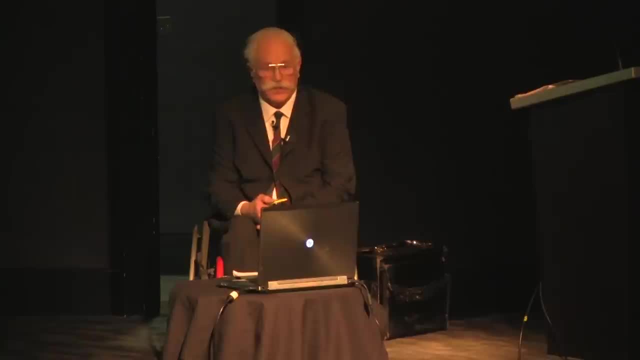 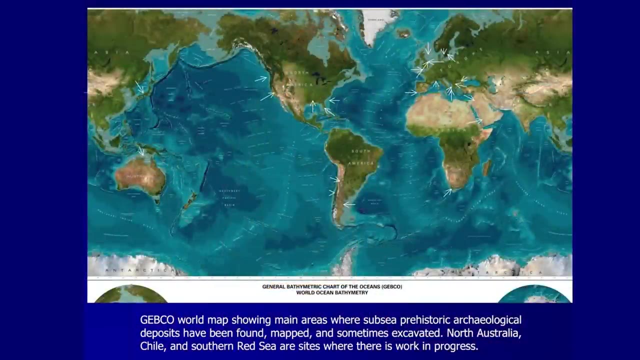 we're generating literally hundreds of millions of dollars of research and research and research, hundreds of papers a year on this subject. again, no mystery. straight to the answer: where are the sites surviving? these arrows show regions where prehistoric sites survive. they're not single sites. for example, in the baltic there's probably over a thousand mesolithic and neolithic villages. 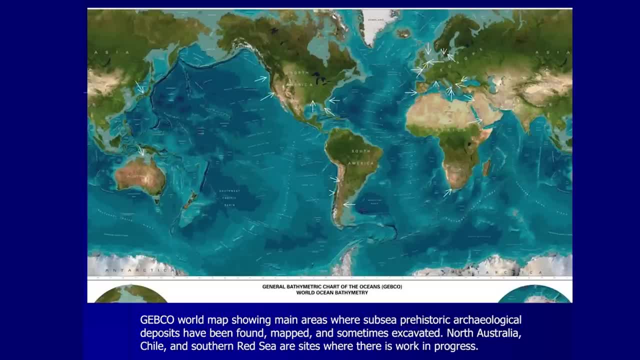 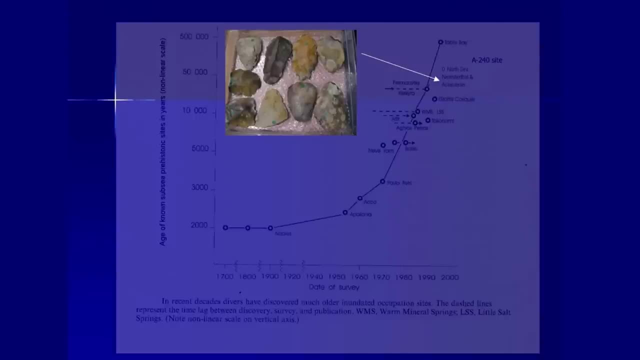 underwater. there's one site down here in cape town. there are hundreds of sites in the mediterranean, many tens around florida and the east coast, usa, just a few in south america. the age of sites against date of discovery, said people knew there were underwater sites, or two or three hundred years ago already, but it's really only after 1900. 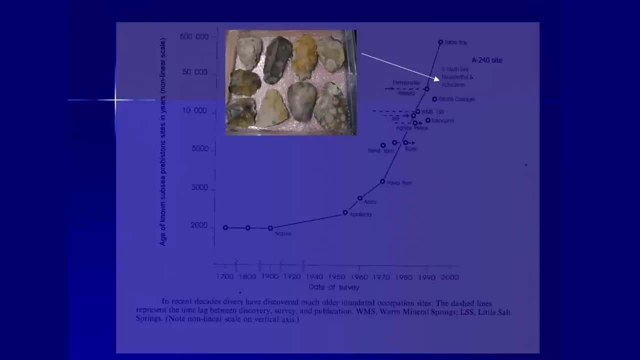 that they start to realize they can actually find sites and date them thousands of years ago. these are the names of different sites that you can look up in the literature or in the transcript which is distributed afterwards, and you can find the references to. most of these sites are on the. 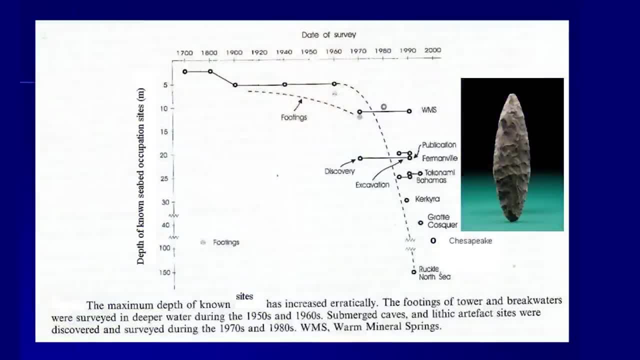 web. if we look at the depth of discovery again, before 1900, it was mostly classical sites and stuff in the mediterranean which had been submerged by earthquakes rather than sea level change. and then, as we come forward in time, deeper and deeper until in the 90s, around about 1990. 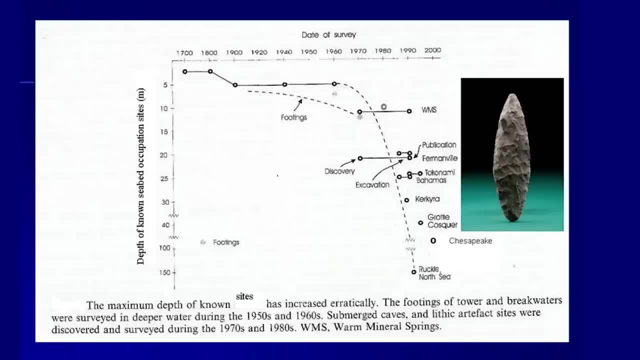 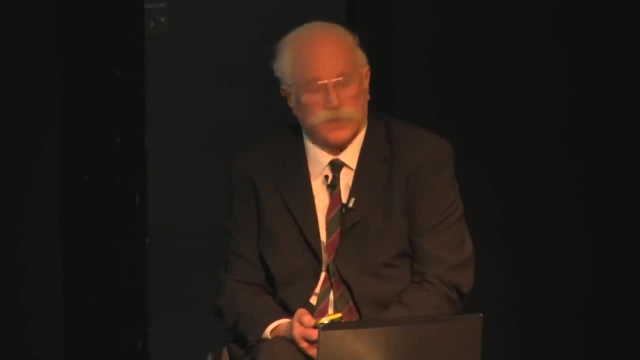 a flint tool was found between the shetland islands and Norway at a depth of 145 meters. This lovely tool is known as the Sinmar flint. It's actually rhyolite. It was found by an American fisherman off the coast of Delaware at a depth of 80 meters. 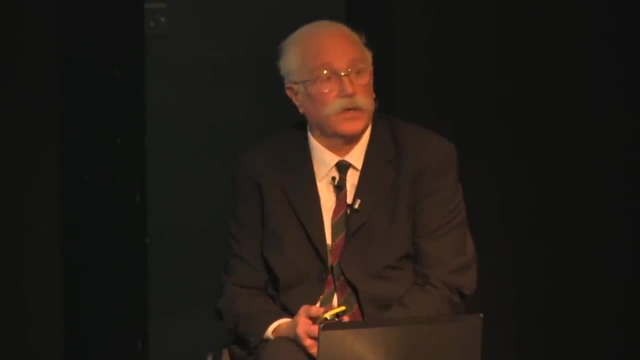 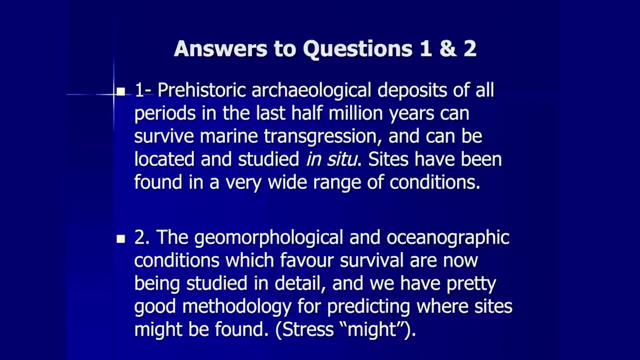 of water, And I think there's going to be an article about it in Antiquity by Dennis Stanford in the next few weeks. Okay, the answers to questions one and two are quite simple. The prehistoric sites do survive, even if they're completely unconsolidated. 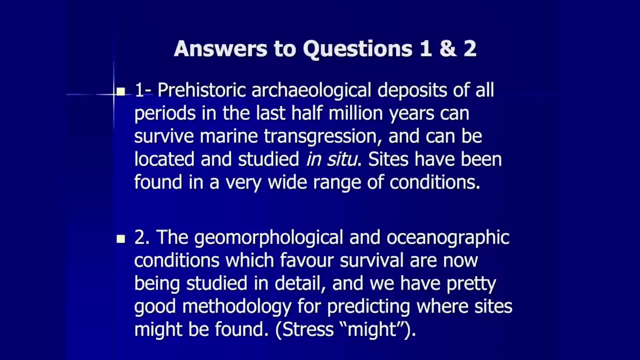 just a Bronze Age village or Stone Age Neolithic settlement, which is just wooden hut posts and flint tools and a hearth or fireplace and so on. They do survive the waves coming over them And we can work out the sort of environment in which they can survive. We can't predict. 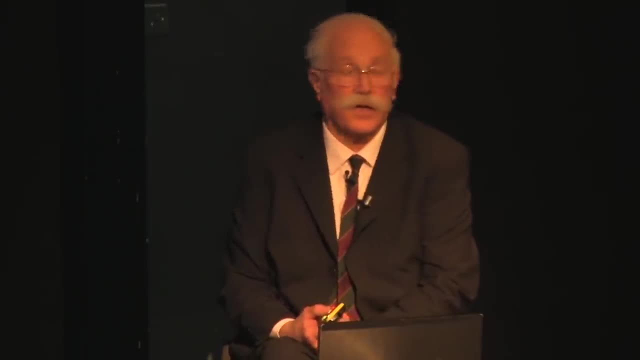 the location of sites Exactly, But we can work out already where there's a high probability And there's a lot of work going on on that. Okay, I'm now going to start looking at sites, and the age is going to increase. We're. 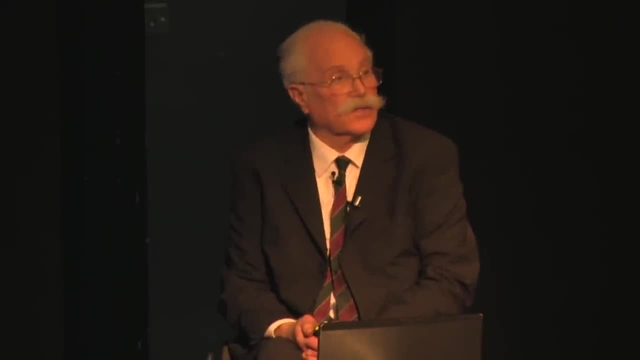 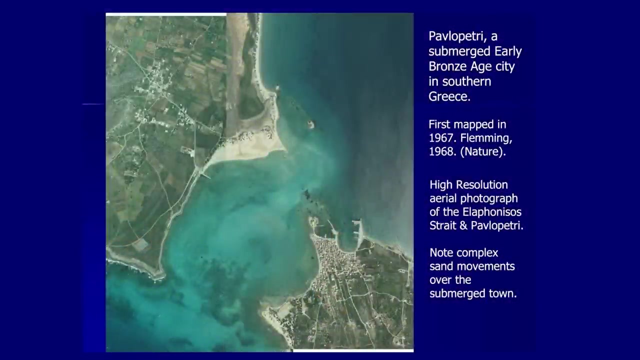 going to start in the early Bronze Age and go back faster and faster until we get to about a million years. This is Pavlopetri. I found this site in 1967 and made a sketch map of it which was published in Nature. 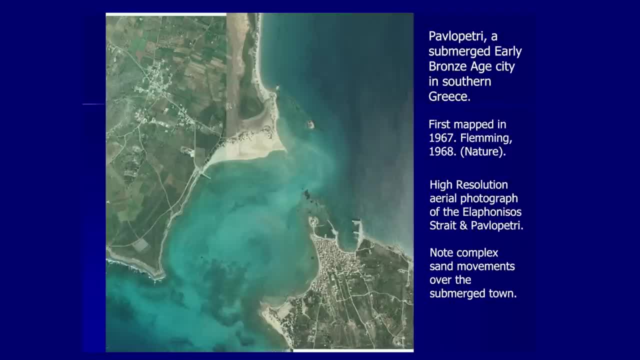 And we then got a team of divers from Cambridge University and, I think, one or two from Birmingham and London And we had a permit from the Efforet of Underwater Archaeology And the resulting map was published in the Bulletin of the British School at Athens in 1969. You can see that there's 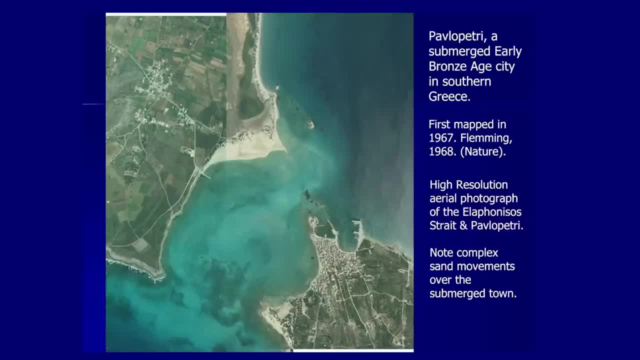 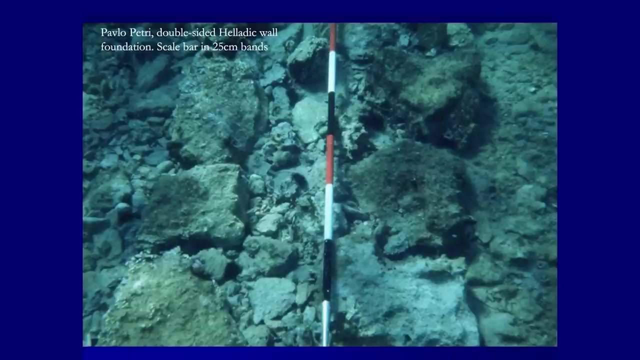 a strong current through here, sand moving everywhere in this channel And the coloration here you can see the sand moving. This is a photograph from 1967.. Kodachrome film. if anybody remembers what that is, The film speed ASA 10.. Again, I doubt if anyone under 30 would know what that means. But there you go, It meant. 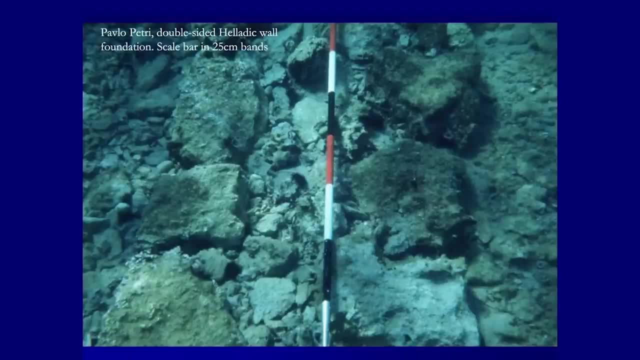 that you had to have an exposure of seconds- Not quite Well, certainly half a second- to get that sort of picture underwater. You can see there that there are lines of stone which are not squared, but they're quite clearly laid in an intelligent way to make a wall which is about a meter thick. These marks are 25 centimeters. 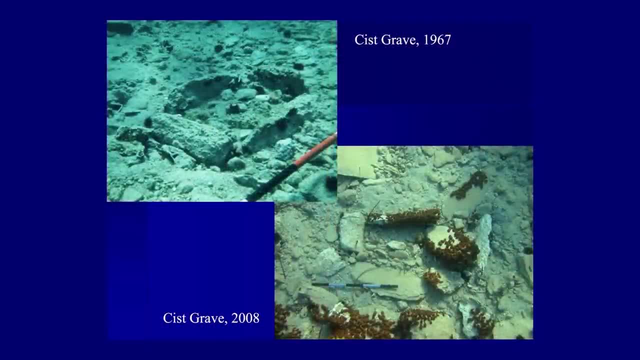 Again: 1967 on the top left and 2008 bottom right. The change in color is partly real. Obviously, some of it could be due to the difference between Kodachrome and modern digital photography, But that shows a perfectly clean seafloor and a box grave. You can see it's about a bit more than half. 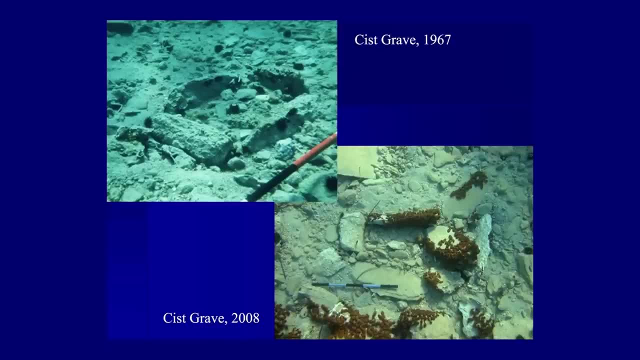 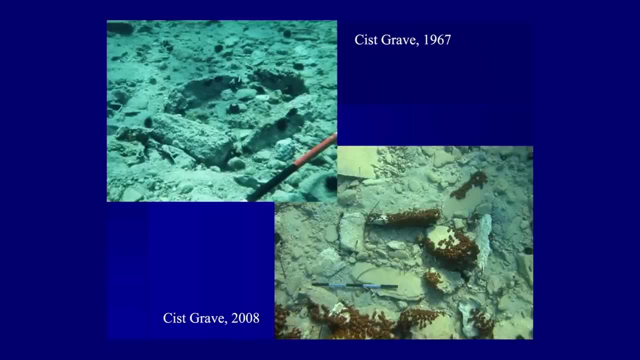 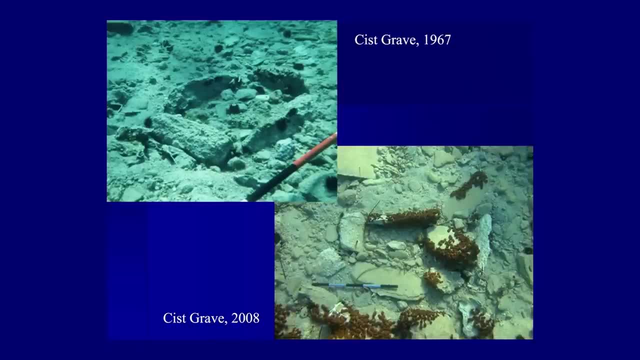 appears to grow up. When the sand's been lying over the city for many years, it's clean. When the sand moves and stays away from an area for a decade or two, you get those boring sponges. Another picture from 2008.. You see a large rectangular room. 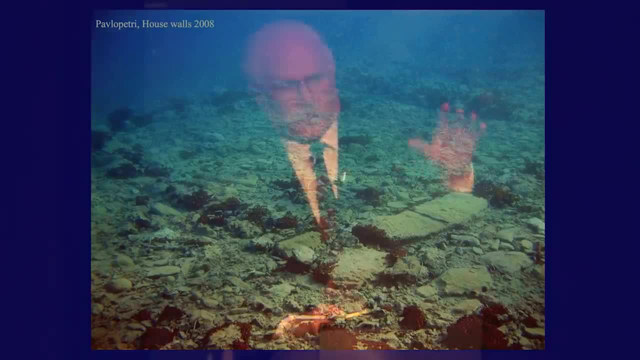 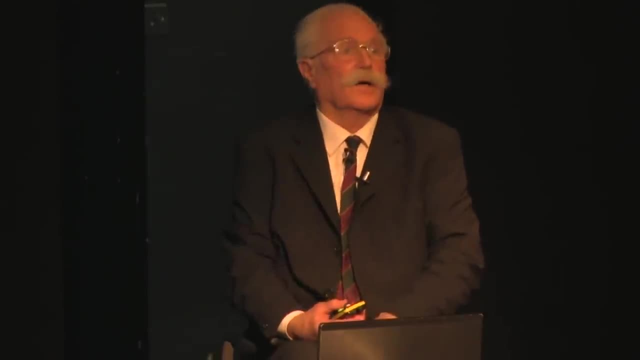 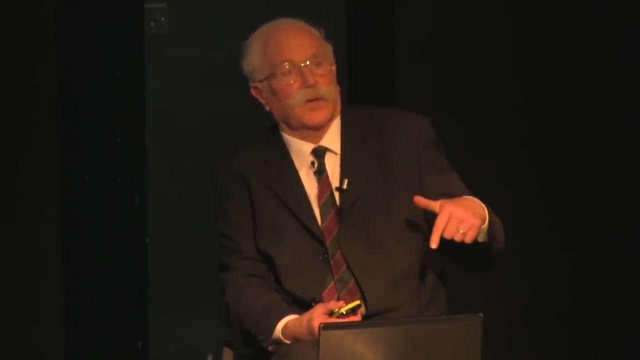 We decided- or John Henderson, who got the permit, in the sense that there had to be a professional professor of archaeology leading the project. So we had a multi-disciplined team from the Hellenic Center for Marine Research, myself from the Oceanographic Institute, people from Australia. 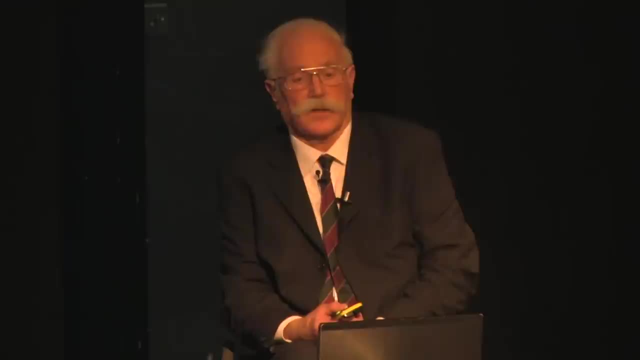 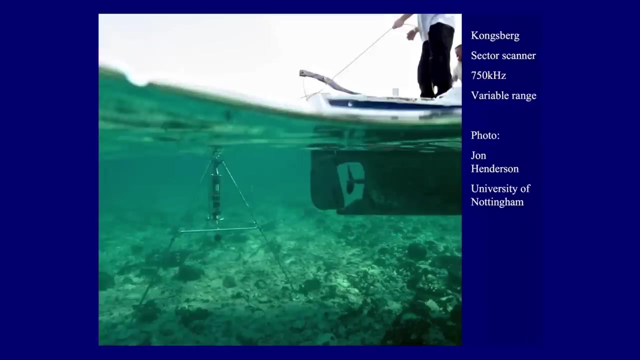 America, a very good team of Greeks and people from other countries working together, And one of the techniques that we were testing was uh sector scanning, sonar. The rotating cylinder there goes around projecting a very high beam, high frequency beam of sound in steps of about a degree, so that you get a complete map of the 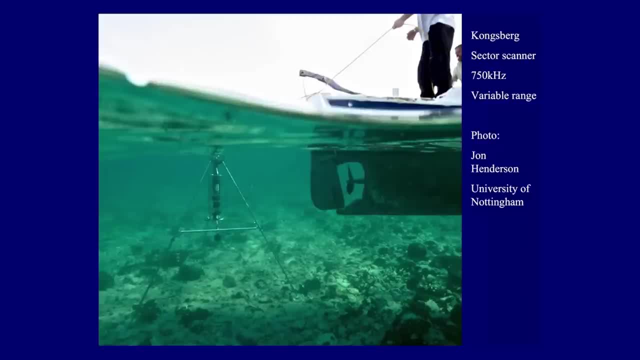 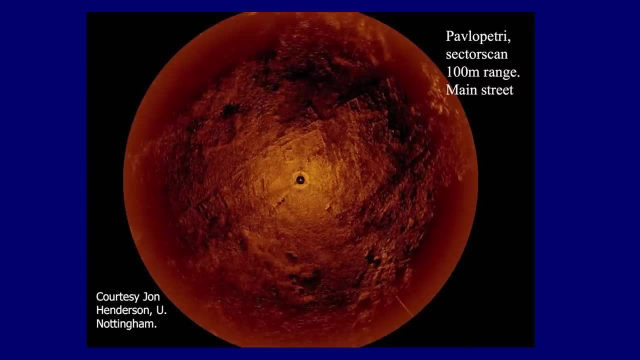 seafloor within 100 meters in a matter of minutes And the resulting map looks like that. This is 100 meter range, So that's 200 meters altogether, And you can see the main city street going through there. And you can see the main city street going through there. 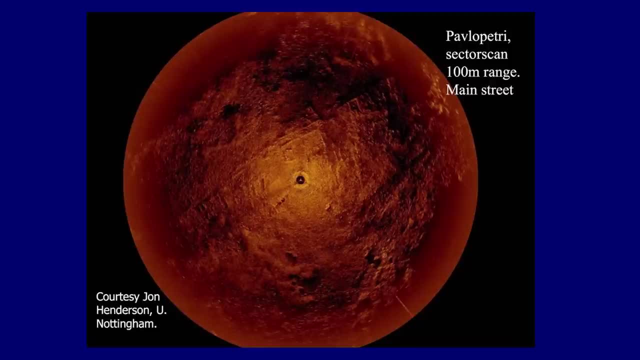 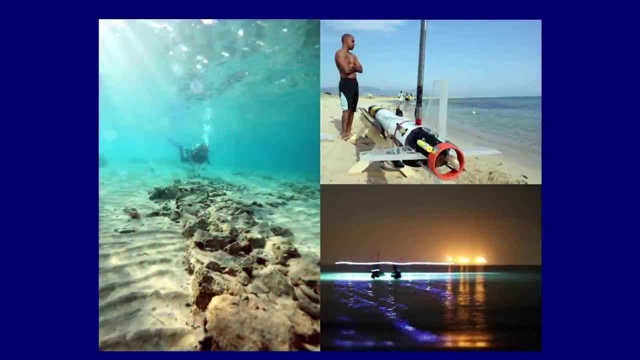 Further research techniques. Obviously, we had divers working all over the place with sketch pads. That's our daughter Kirstin there and over, swimming over one of the big walls. She was the chief architect for the project in one of the years between 2009, 2011.. 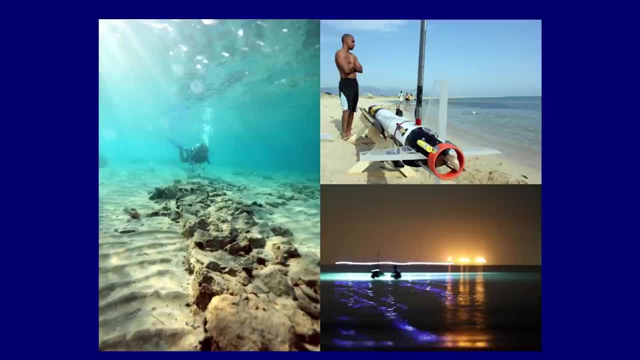 She was the chief architect for the project in one of the years between 2009,- 2011.. was developed specially by Oscar Pizarro from Australia. He has a special unit working on digital robotics for imaging earth sciences, And the vehicle has been adapted. 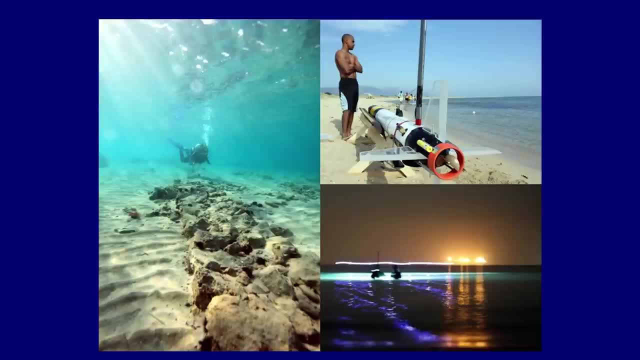 so that there's a GPS sensor on the top there and it can be programmed to navigate backwards and forwards with a spacing of one or two metres over the site in a scanning system which is completely accurate and would drive any divers absolutely bonkers. You can't imagine people swimming backwards and forwards. 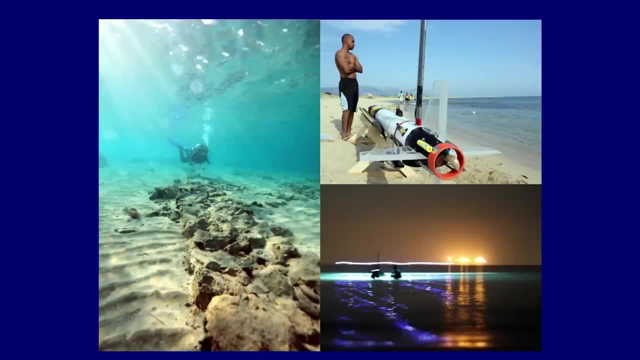 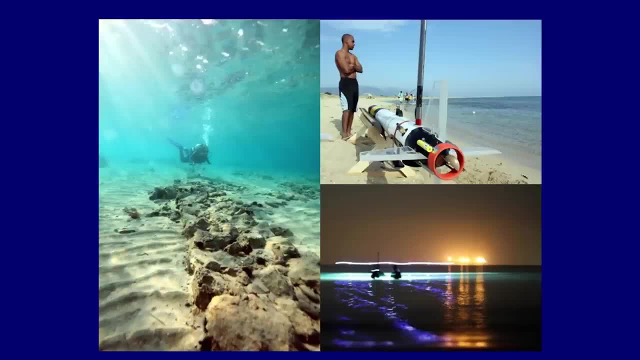 is fitting together thousands of images and adjusting them continuously to get the best possible fit, And the ripple patterns confuse the software. So we did it at night And, because the whole thing is with flash, a few nights where you've got very accurate photographs. 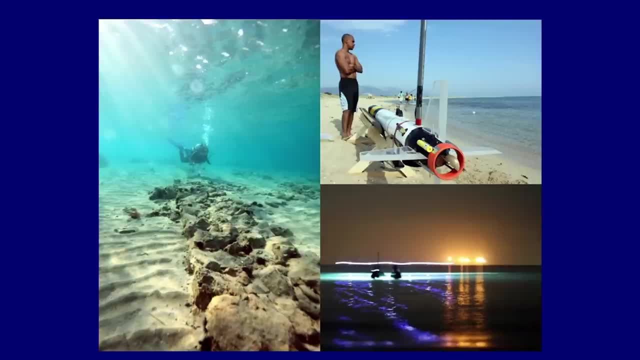 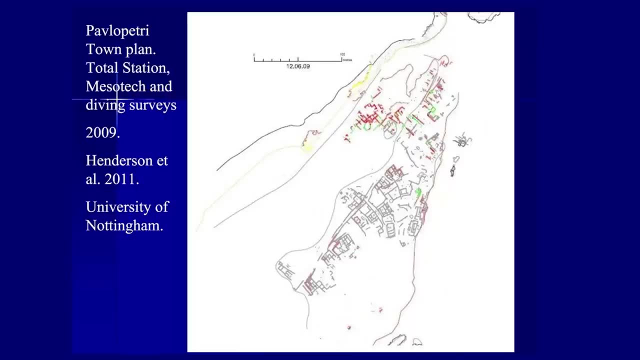 and produced an extremely accurate map of the city And there you can see that diagonal street which appeared on the sector scanning map. A lot of the. This is reproducing rather more accurately the map which we made in 1967, 68.. 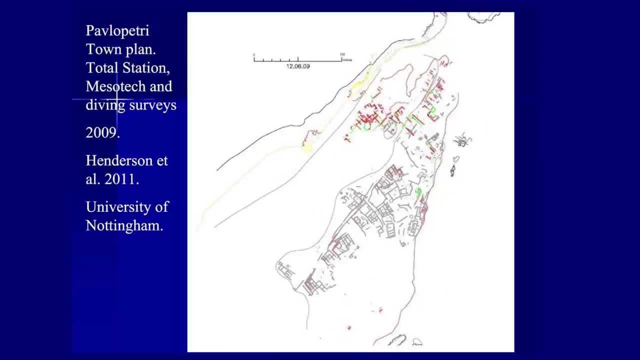 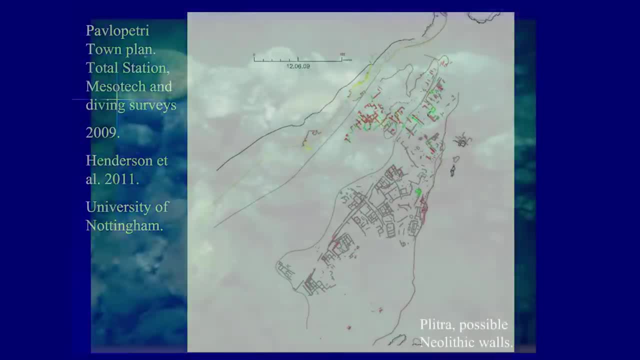 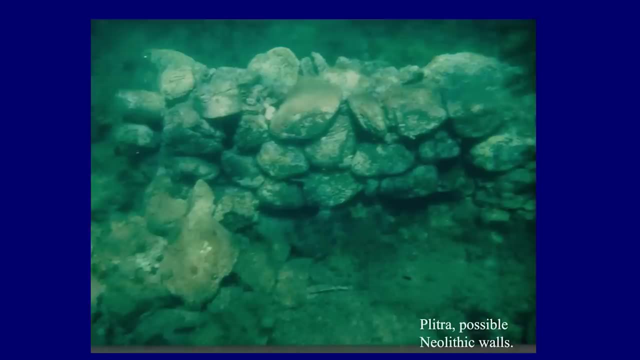 But all this area was discovered new and had been revealed by movements of the sand in 2009,. 10. Just north of Pavlopetri is the site of Plitra, which I think is possibly older. The oldest pottery found at Pavlopetri is just Neolithic. 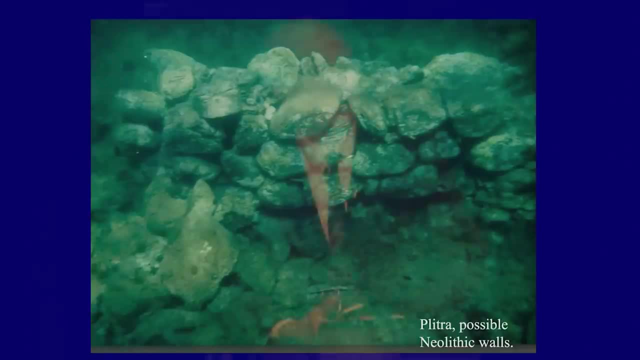 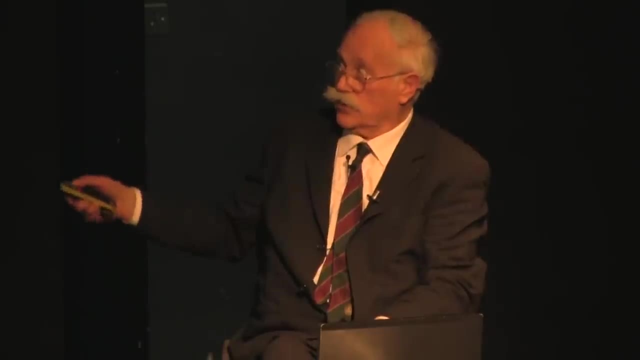 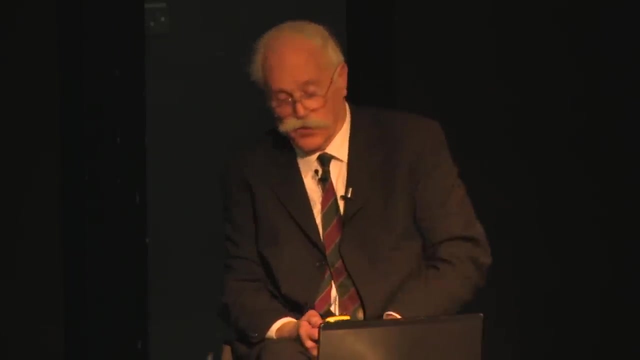 late Neolithic, perhaps 5,000, 5,500 years old. This site has got standing walls. You can see that the stones are not shaped. Nobody has ever been back there to map this since 1967. I don't know why. 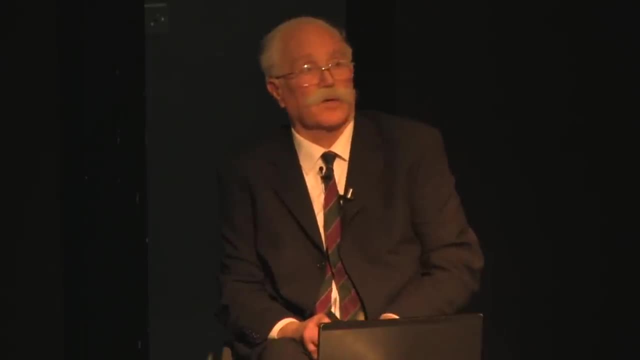 It seems to be a very interesting site and could be one of the oldest and most complete Neolithic suburb sites in Greek waters. Okay, we're going back now to 5,000, 6,000, 10,000 years And we need to start looking at sea level change very quickly. 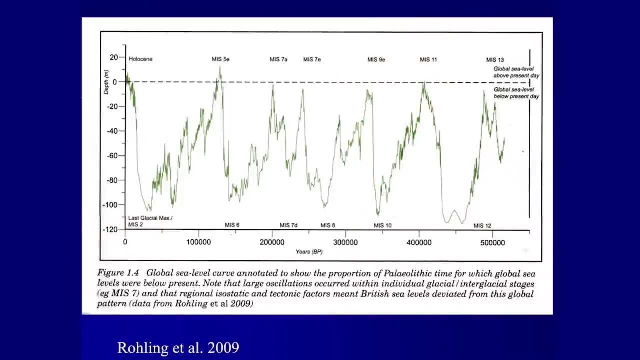 Very seriously. During the last half million years there have been repeated ice ages about every 125,000 years As the ice For the moment. I'm going to go forward in time. As the ice builds up, the sea level drops. 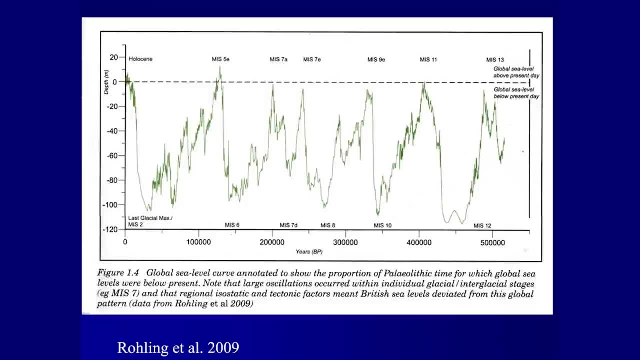 down to about 130 metres and then the ice melts relatively suddenly and the sea comes up to the present sea level. If you look at the last glacial cycle, the sea level That spike seems a bit high. The sea level was about 5 or 10 metres above present. 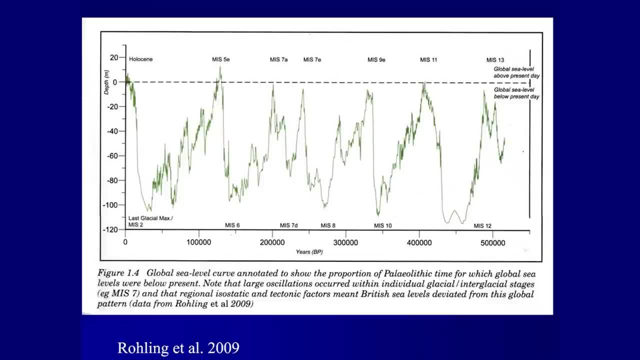 at the last interglacial. It dropped in a series of cycles, driven by what's called the Milankovitch astronomical cycle, And then the sea level rises very rapidly from 20,000 years ago up to about 5 or 6,000 years ago. 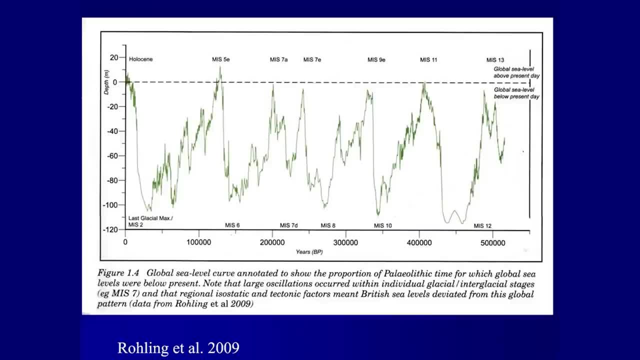 So for the next few minutes we're going to look at that slope going backwards to 20,000 years, And as the talk progresses we'll go right back through all these glaciations. I'm sure you've seen maps like this in the popular scientific journals. 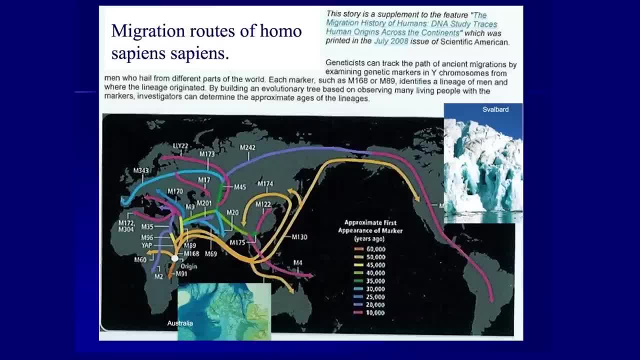 the DNA data on human migration And you can see obviously that people are crossing sea channels all over the place. On this map they have not suggested that people cross at Gibraltar or Tunisia or Sicily, but the Southern Red Sea getting into Australia. 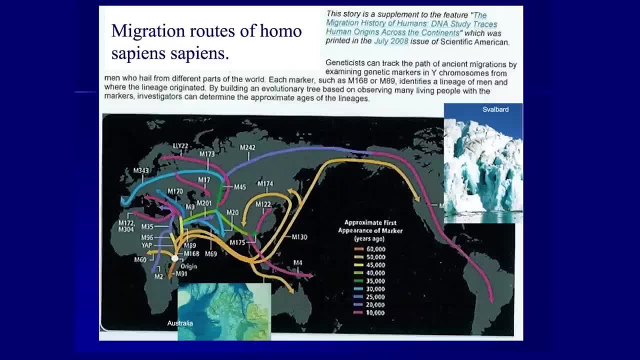 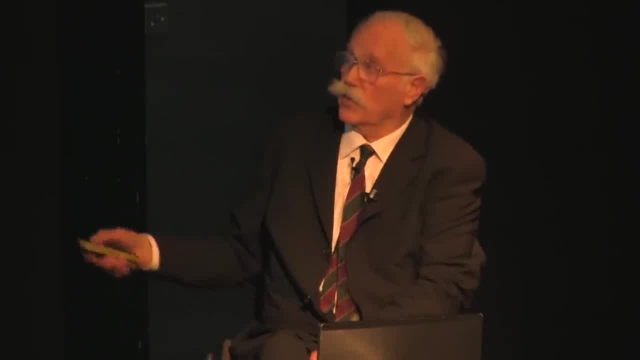 which was never connected, Even at low sea level. Australia was not connected to Southeast Asia and crossing here at Beringia. I have a sort of love-hate relationship with people who do this work because obviously the DNA information is staggeringly important. 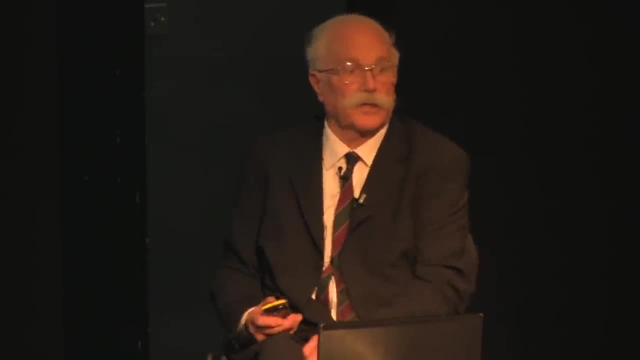 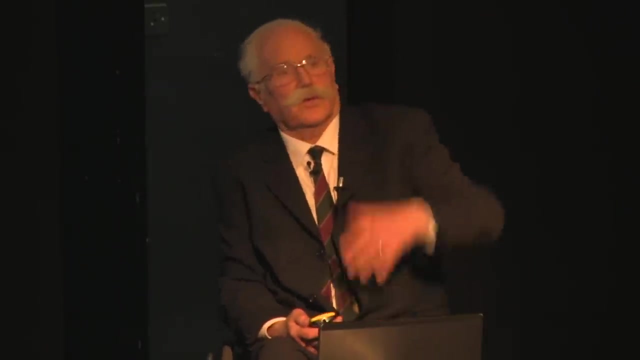 But this kind of map is what I call the broad brush brigade. You take a big coloured pen and you put an arrow like that, sweeping across a huge geographical area. I'll come back to this topic in a minute. OK, if we look at the European waters, 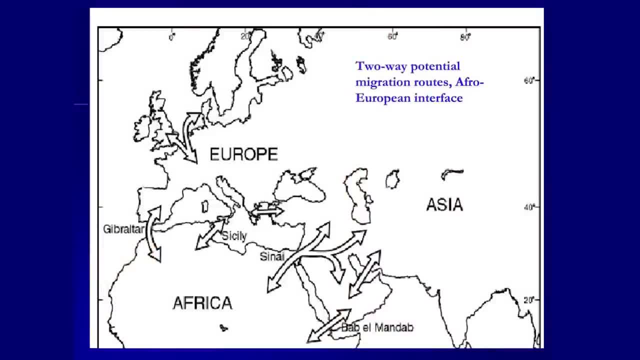 these are all the key crossing areas And the occupation of the British Isles. the oldest occupation of Britain is at least 850,000 years ago, near Lowestoft. I'm not sure why, but the people were living there almost a million years ago. 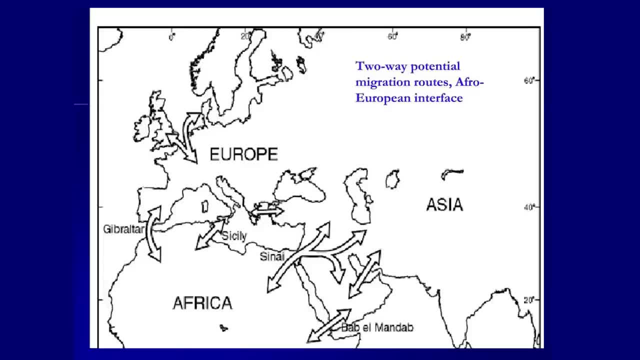 and it may be even older. This is the oldest site north of the Alps. The crossing areas- I've marked them with arrows, both ways. People were crossing both ways And almost certainly if you lived on the shore, you had people who were skilled. 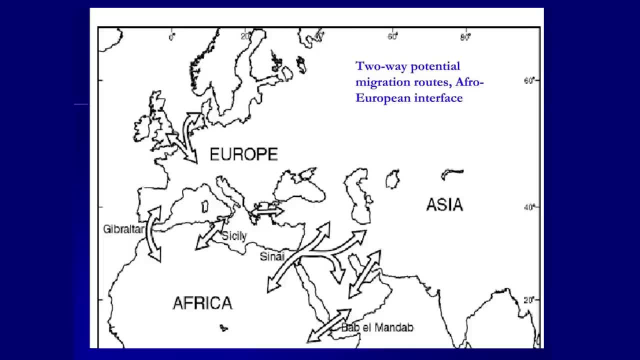 like fishermen today and knew the channels and knew the currents, And they went backwards and forwards, as it were, just to see their brother on the other side for tea, and came back again. That's not a migration. You've got population on this side. 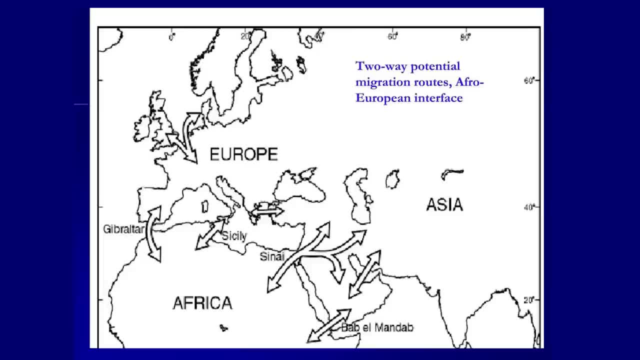 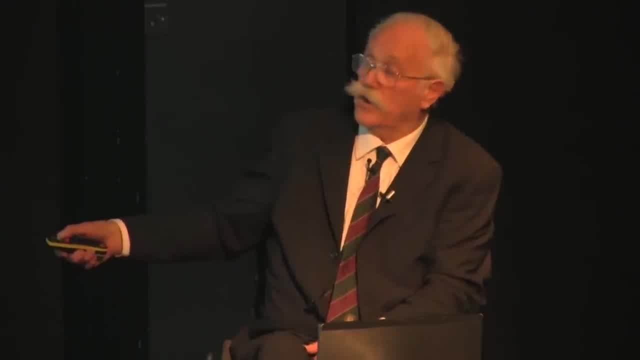 a much thinner population over here and over a few thousand years, because the climate changes on one side or population increases. only ten people that go that way, only five come back And we call that a migration, Typical migration, say from Africa to Beijing a million years ago. 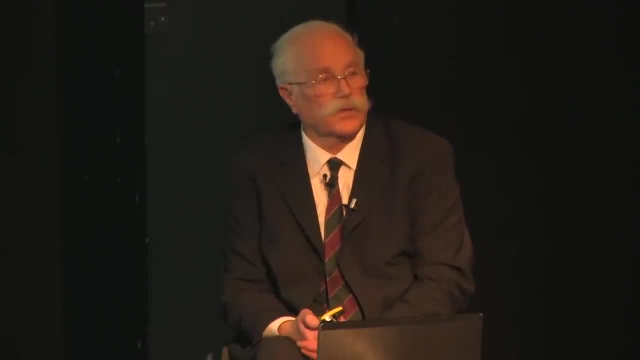 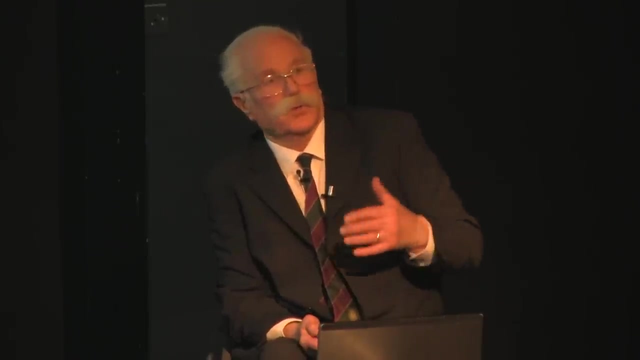 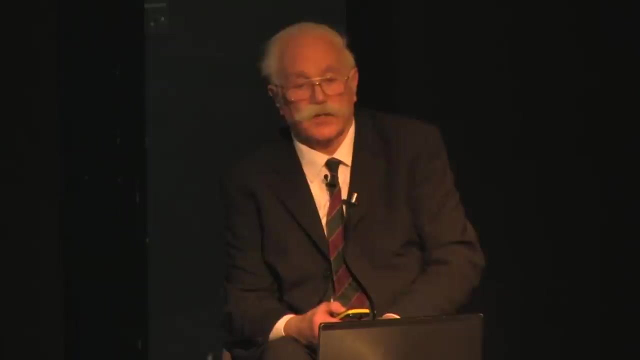 took place probably substantially slower than one kilometer a year. So we talk about migration very often, but really it's a slow ecological diffusion in which the hunting area or migration area with the seasons just slowly changes Year by year. A quick runaround sites in different areas. 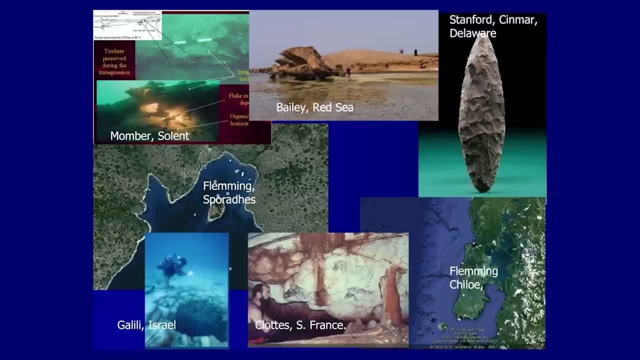 A submerged site in the Solent, about 8,000 years old, at 11 meters. The Red Sea- I'll come back to that again later. The Sinmar Flint: 80 meters of depth, over 20,000 years old. 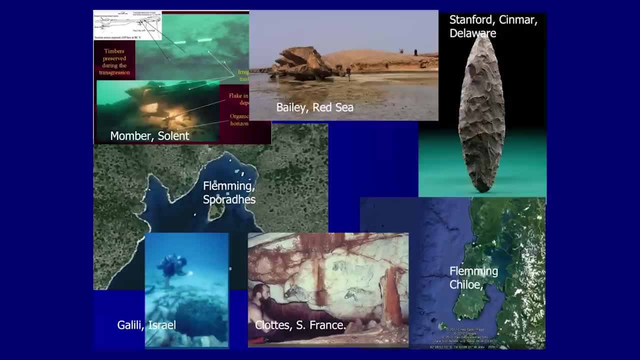 and about 100 kilometers off the coast of Delaware. The site here, Monteverde, has been about 14,000 years old and I've been looking at the seabed geology here and other sites corresponding with Diego Canabrias. 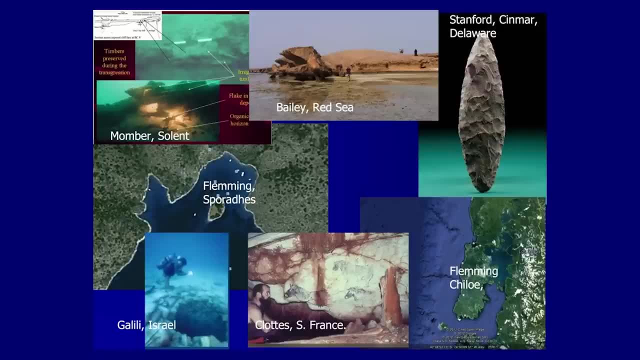 who was in Valparaiso, Caves underwater with paintings, a well in Israel and a freshwater site going down 15 meters below sea level in Atlit, an island in the Sporades which we'll come back to later. 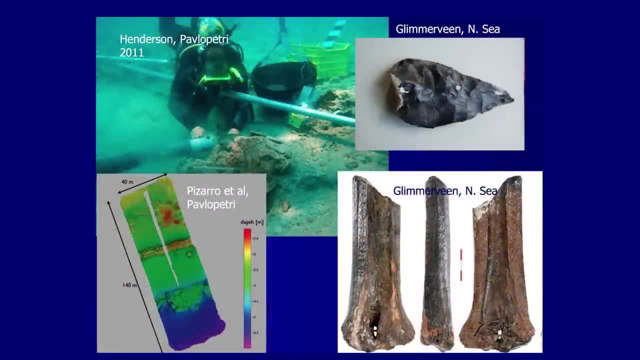 And again work underwater. at Pavlopetri flints from the North Sea, the beautifully shaped Acheulean hand axe, the sort of mapping that we can do with that autonomous underwater vehicle. And this which I love particularly is an exquisitely carved bone. 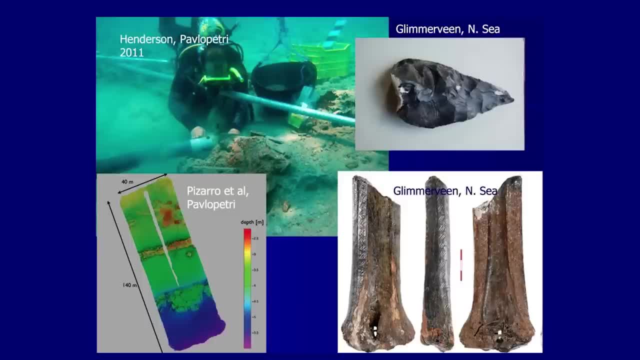 from the central North Sea, about 11,000 years old, And looking at this pattern, you can see that somebody just did that for pure joy. You can see somebody sitting in the sun 11,000 years ago and inscribing this for no function. 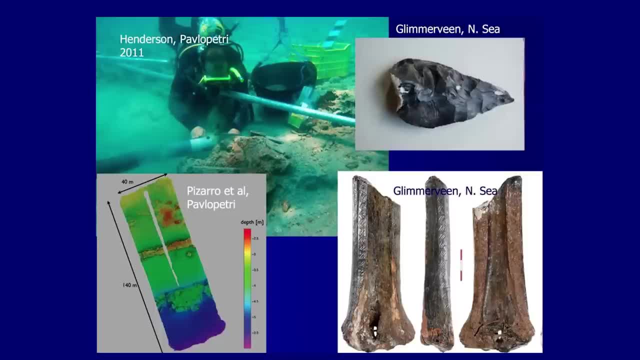 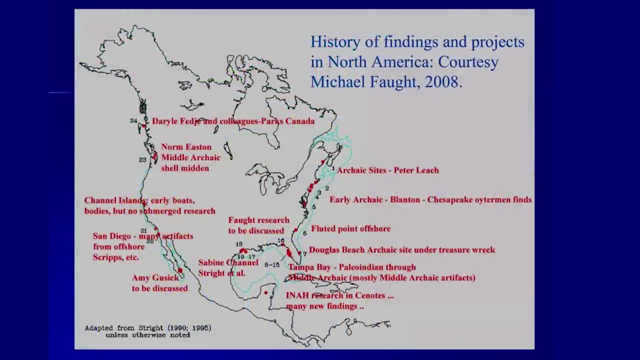 It's probably a knife handle or something like that and just showing their skill to make a beautiful tool. Still in the same date range, before 20,000 going out to the USA, Mike Fort has provided this map and the data on the rise of sea level. 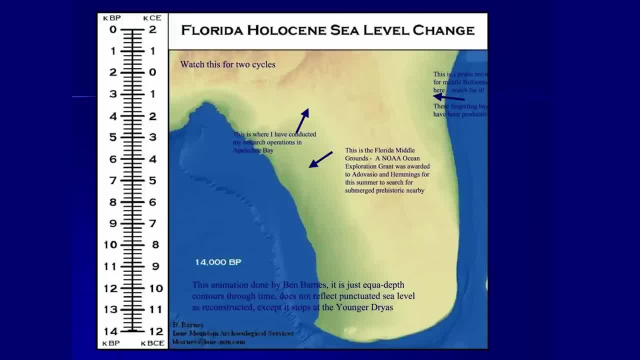 around the Florida coast. Yeah, there you go. the sea level's coming up. The continental shelf in the Gulf of Mexico was extremely well protected and very, very shallow and very low gradient, So there are paleo-Indian sites going way out into the Gulf. 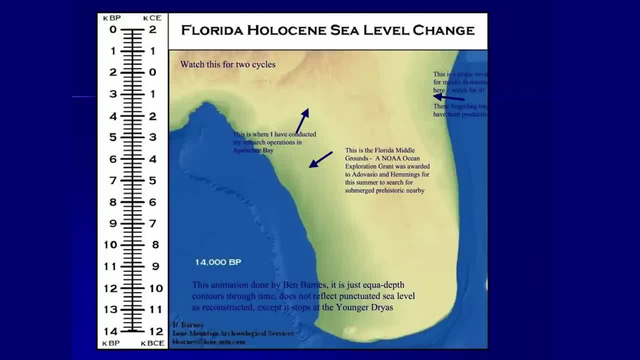 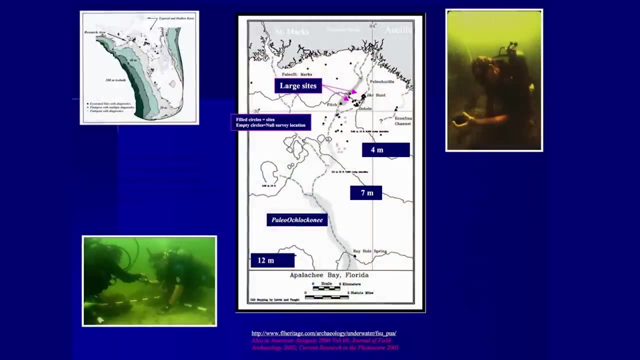 and sites have in fact been found on both coasts. Even on the Atlantic coast, where you've got the sea pounding in the gentle shelving sandy beach, protects prehistoric remains underwater. This is Mike's work in the Gulf and you can see that he's finding prehistoric sites. 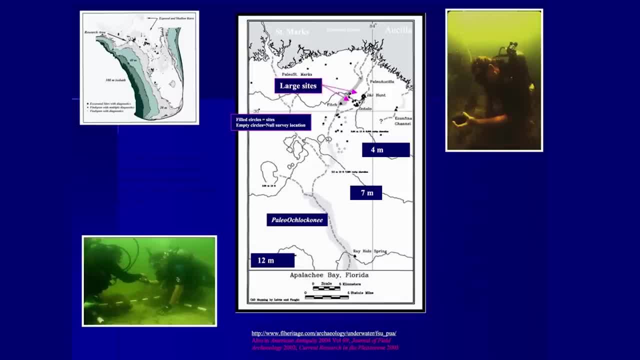 Tens of kilometers out into the Gulf of Mexico, very, very shallow gradient, down to a depth there of 12 meters. There's a book coming out, published by Springer. The final proofs went to press today. I don't know how long these things take. 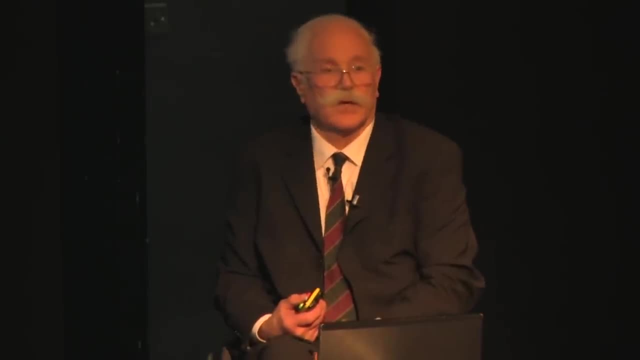 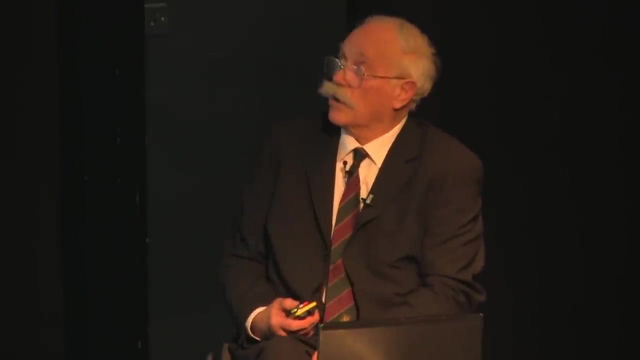 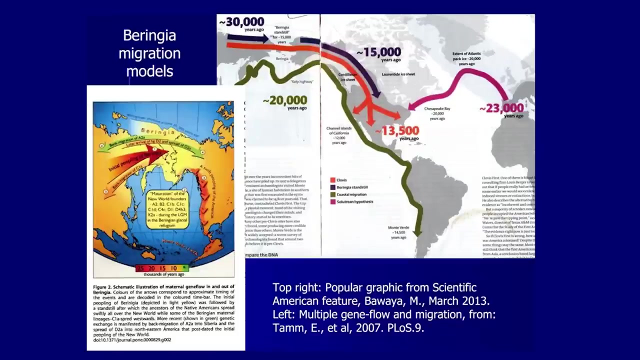 to publish in the modern electronic age, but I would guess it would be on the web or on bookshelves within a very few months. We're back with the broad arrows again. I prepared this slide for a talk in Poland at the end of last year. 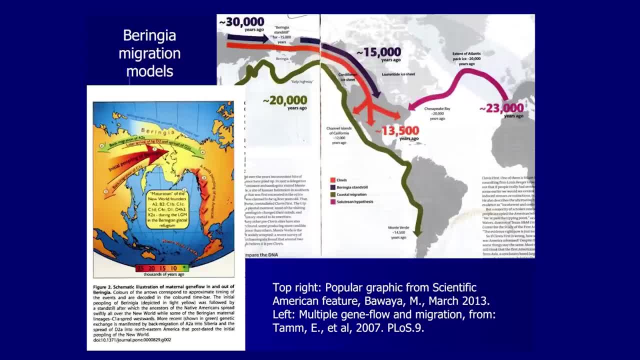 intending to show the difference between popular magazines, scientific magazines and serious scientific literature. These are the sort of what I call Napoleonic view of migration direction or whatever. It's not a lie, I mean. these dates are correct, substantiated by very good 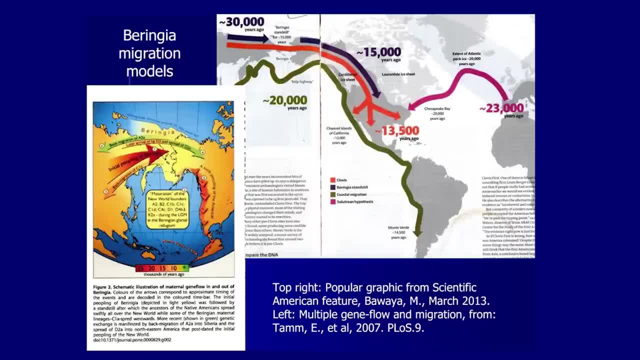 scientific research, but this is not how people move. This is not how migrations take place. I then did a lot of research in the literature on DNA and human genetics and so on, and look at that one That looks like the opening scene of Dad's Army. 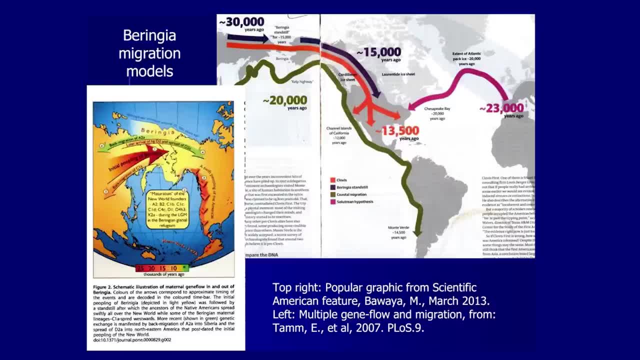 you know the one with all the arrows. They may take this out of the tape afterwards, but I can't resist it. I mean, really that is not serious archaeology, And that's. I did a scan through about 50 articles. 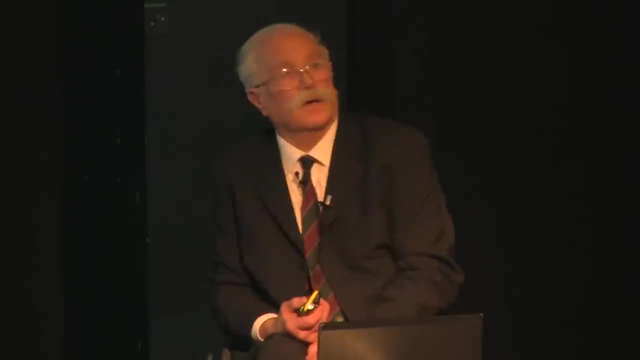 in this literature: DNA, genetics and human evolution. One paper mentioned the terrain. One paper, which was about migration around southern India, mentioned that if you Sea level drops and you've got exposed limestone, coral reefs, it's not that easy to migrate fast. 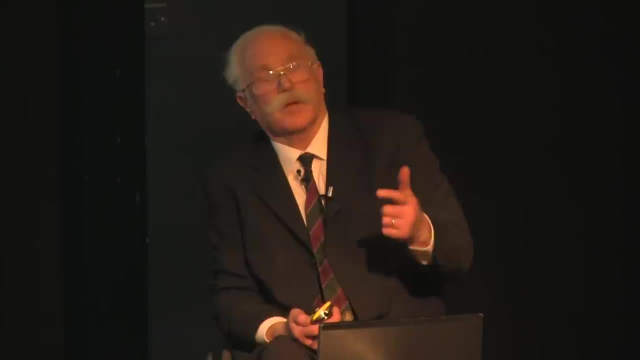 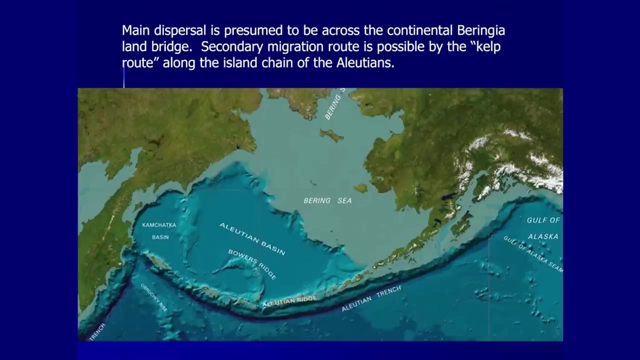 Nobody else paid any attention to the terrain, the climate, the water supply, the vegetation, the food or anything else. OK, Migration into America, The Bering Straits: here Some work has been done, really pioneering research there, but one of the key issues is whether people walked across. 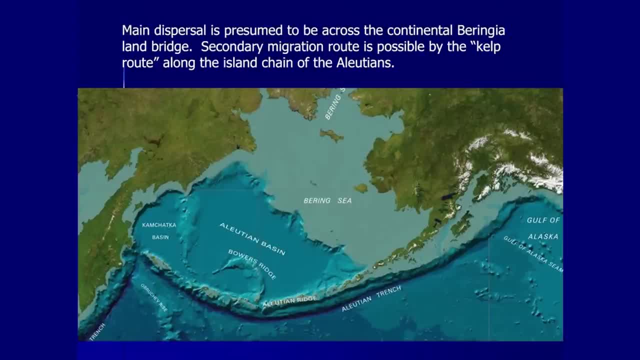 the tundra area when it was glacial, or whether they came or both, whether they came through the Aleutian Islands by boat, And I wanted to check whether the island topography here has been roughly similar for the last 20,000 years. 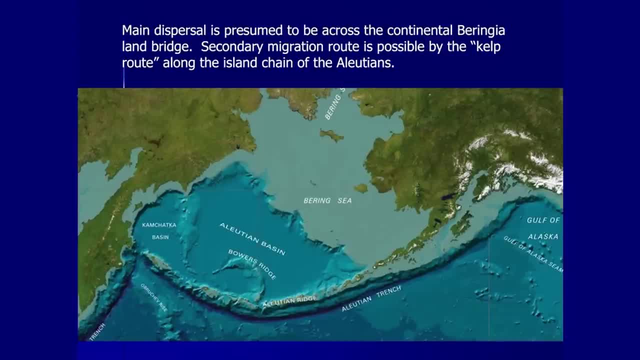 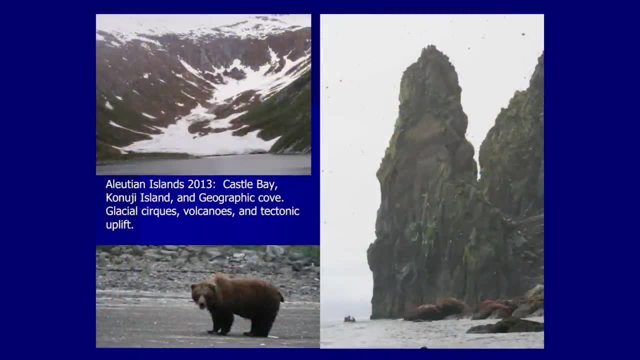 or whether the land has been coming up either due to tectonics and plate subduction or the removal of the weight of ice. So Jay Kleinberg and I took a boat cruise from Kamchatka to Seawood in Alaska and looked at a lot of these islands. 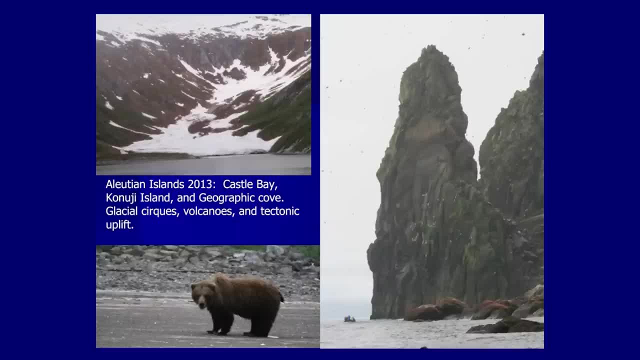 We landed with zodiacs And you can see it's a pretty rugged terrain. There are glacial cirques everywhere. The glaciers obviously melted a few years ago, Incredible volcanics on these different islands and a lot of wildlife. It's a pretty rugged place. 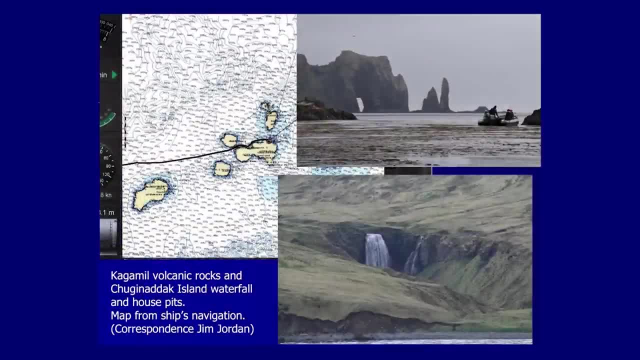 More of these volcanic islands and pinnacles. Again, the base of a volcanic cirque- sorry, of a glacial cirque- and a waterfall, And one of the guides on the ship found a hut, a house pit here, but we were unable. 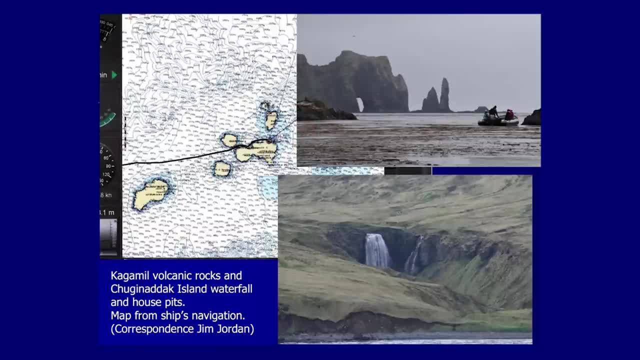 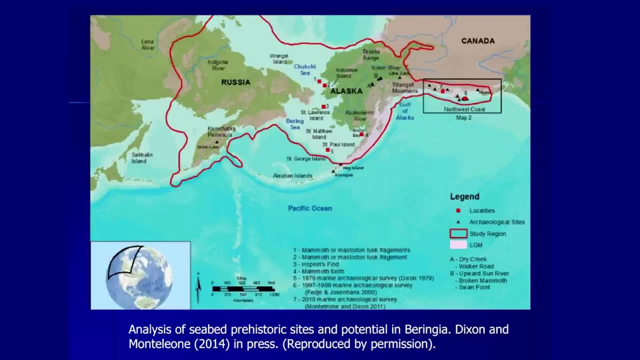 we didn't have enough data to date it and obviously we couldn't excavate. This is from the Springer book which I referred to earlier, which I hope will be published in a few weeks or months, And the work by Dixon and Monteleone. 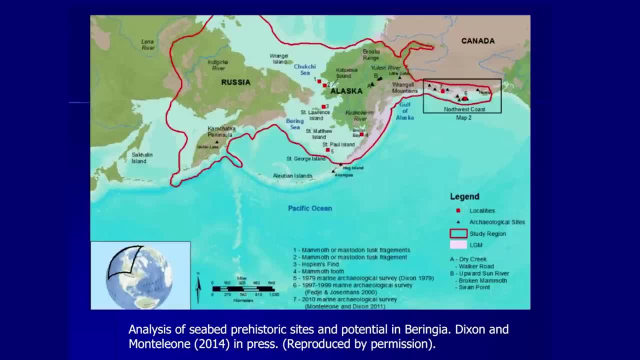 shows how they are gradually building up the picture of archaeological sites in the area. And what seems to have happened- and the DNA confirms this- is that, because the glaciation is always on mountains, you don't get a thick ice cap in northern Siberia. 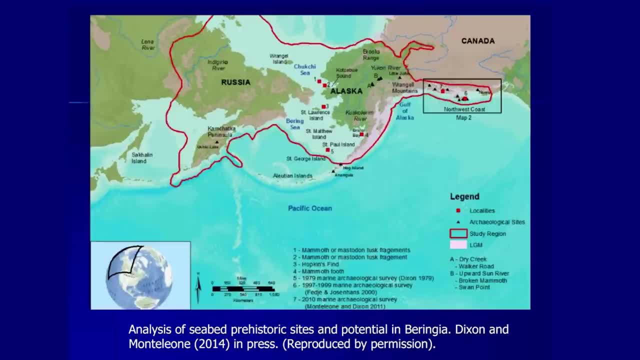 or in northern Alaska, because there's no mountains, as it were, to anchor the ice, And the result is that you've got thick ice here in the Ice Age and the northern part of Alaska was not glaciated, So people seem to have moved, as it were, across the strait. 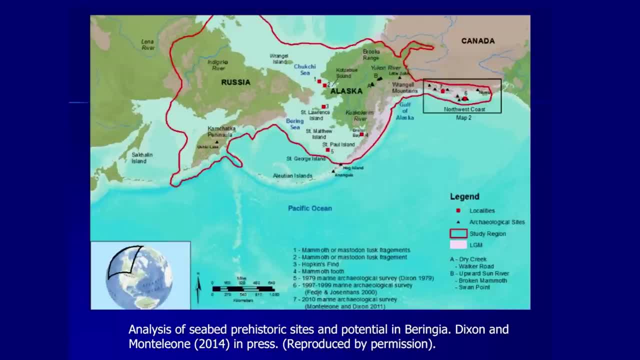 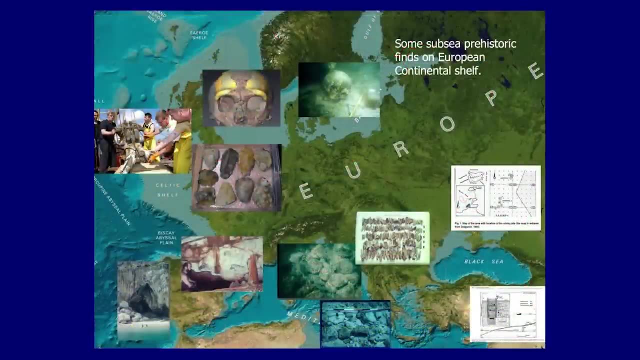 and there was a population here long before they could get down into the main Americas, And then one of the models is that they came down the island chain Back to Europe. Sites everywhere, The Baltic, as I say, well over 1,000 sites in the Baltic. 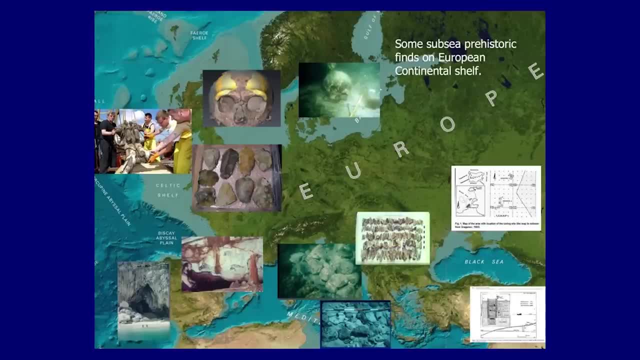 Neanderthal skull fragments from the North Sea. Several more have been found in the last few months: Shirlian hand axes, bits of mammoth walls, bones, the well in Israel, caves in Gibraltar, Human material everywhere underwater. The ice sheets covered Scandinavia and northern Scotland. 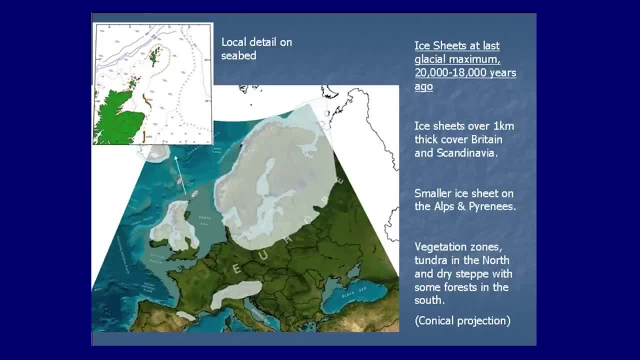 and at different times, the ice actually joined up over the northern North Sea, But apart from that, all this grey area, including the Adriatic and large parts of the Black Sea, were occupied by people. You can see models of the way the sea rose. 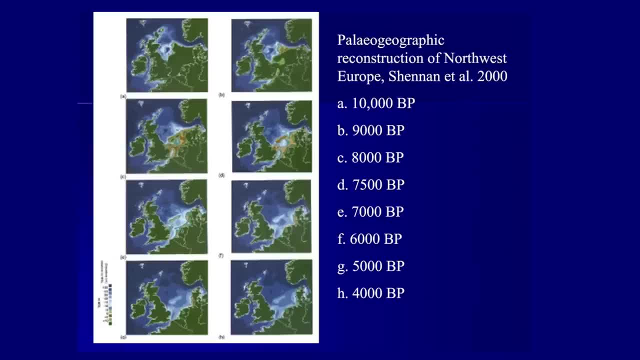 over the British northwest shelf around Ireland and into the Chatham Islands And that's the sort of maximum land area, And then gradually the sea floods in and goes round the Dogger Bank and so on in stages And the press seems to pick up on the Dogger Bank. 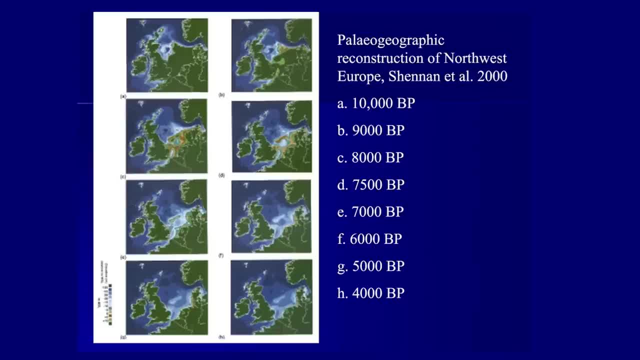 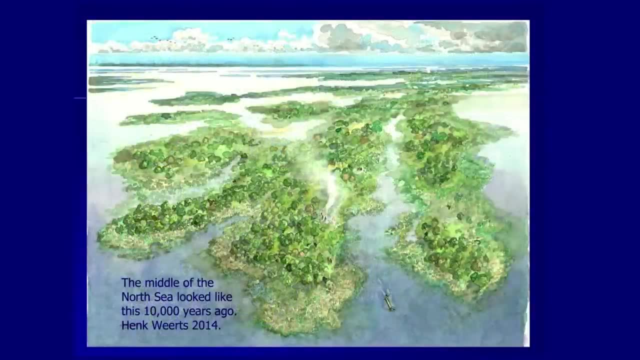 and Doggerland quite frequently, as if it was a high hill with Neanderthals sort of standing on it signalling for help as the water comes round their ankles. They were not stupid, Believe me. The terrain probably looked like that. This is a reconstruction from some Dutch work. 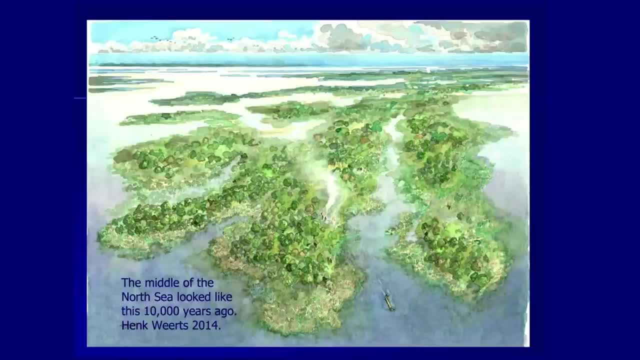 in the last year or two during the excavation of the new Yangtze harbour, And the total relief in the North Sea is about 20 or 30 metres. in hundreds of kilometres It's really just an undulating plain, And as the sea came over you would have had mile after mile. 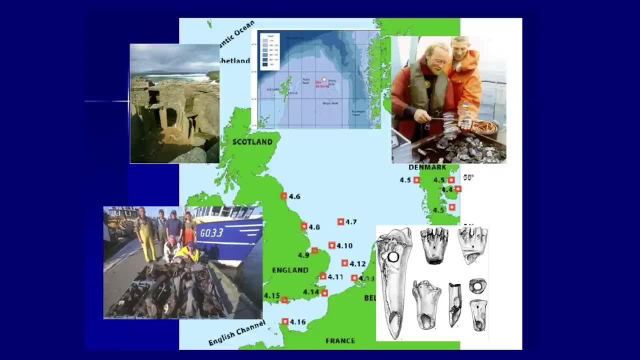 of marshes like that. Sites have been found all round the North Sea, Orkney and Shetland bones coming up with the Dutch trawlers. They find about 10 or 20 tonnes of megafauna bones every year and quite a few worked flints and implements. 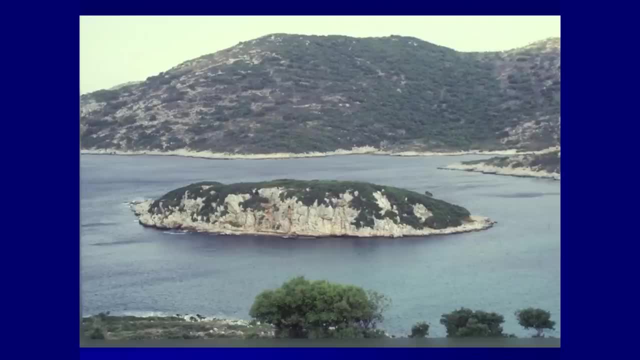 Back to Greece, Iospetros in the Sporades, again around 10,000, 20,000 years, But the site here is 10,000 years old. Nikos Efstratiou and Cathy Giangrandi invited Jay and I. 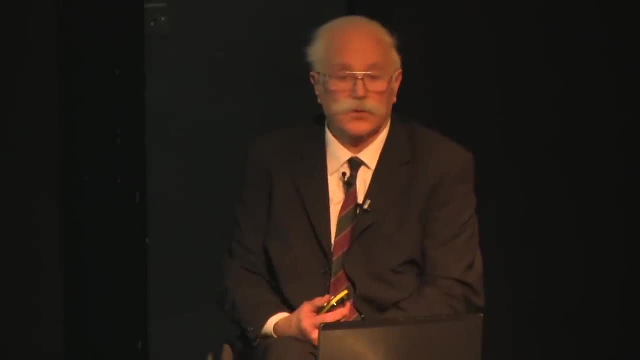 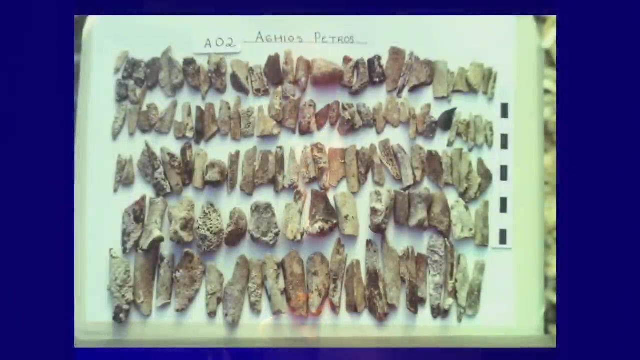 to go out there in 1981. And to cut a long story short, after a while we found a site where you could put down a one-metre quadrat, take five centimetres of sediment off it and you ended up with nearly 200 goat and sheep bones. 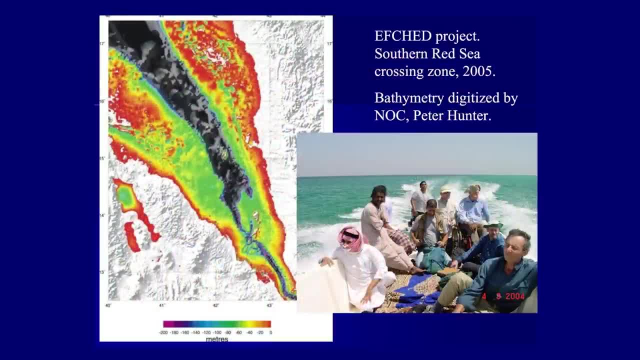 The Red Sea. going further south, right down near Bab el-Mandab, the crossing of the Red Sea, again at low sea level, seems almost certain. The Broad Arrow Brigade now routinely draw arrows across there, although there's no evidence on the ground for it yet. 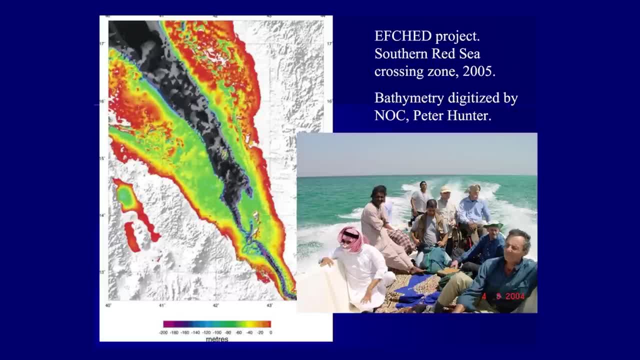 It fits and it makes sense, but that's not quite the same thing as having archaeological evidence on the ground Starting in 2004-2005, Claudio Vitefinzi, Jeff Bailey, myself, Laurence Moran and Abdullah al-Shareq and others. 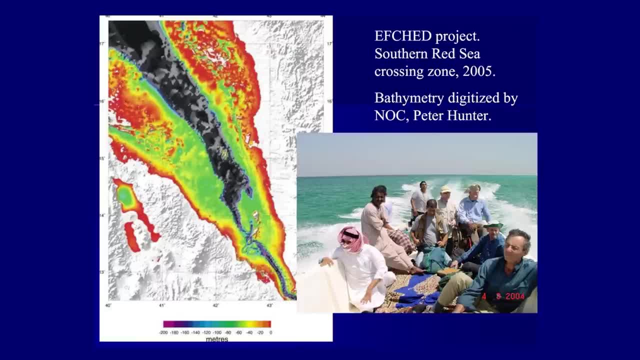 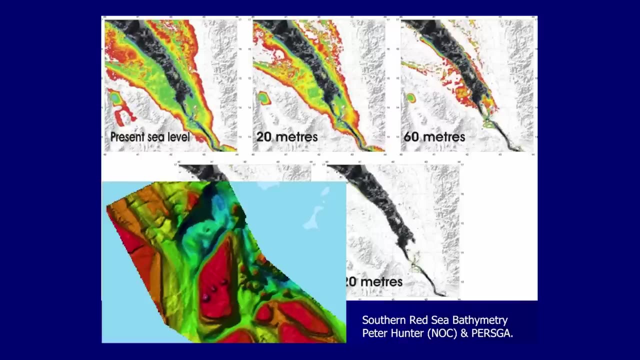 we started looking around these islands and have built up. a place we're looking at in most detail is there is the Farasan Islands. Those are the Hanisha Islands there, Modelling the sea level rise, or rather running it backwards- that's what it looks like now- and as you lower the sea level, 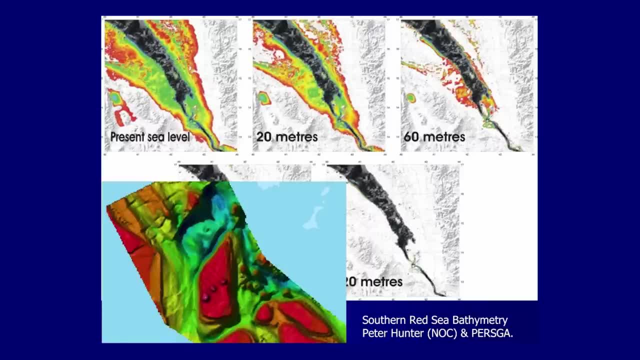 the channel here gets narrower and narrower until there's that tiny little bit there just by the Hanisha Islands. This is a very recent bathymetric survey of that channel showing dramatic graben fault down there. Diving around the Farasan Islands, we used Trimix. 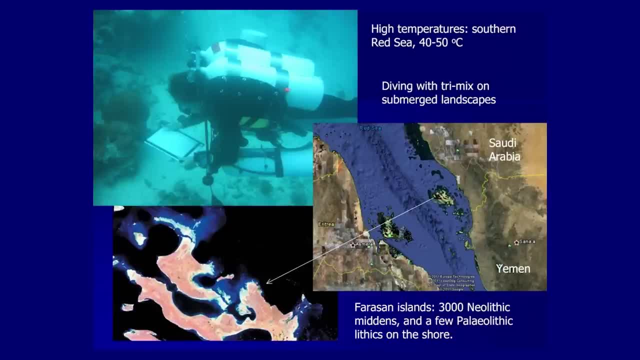 oxy-helium-nitrogen mixtures to dive down to 60, 70 metres, and the extraordinary shape of the islands is due to what's called salt tectonics. As the Red Sea dried out, several times the layers of salt formed. 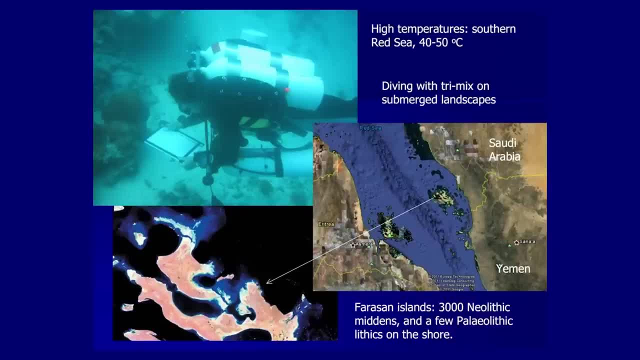 and then rock came on top and then, as the salt leached out, you get these extraordinary collapse features, which can go down 500 or 600 metres, and they would have been lakes, probably freshwater lakes, during periods of low sea level. 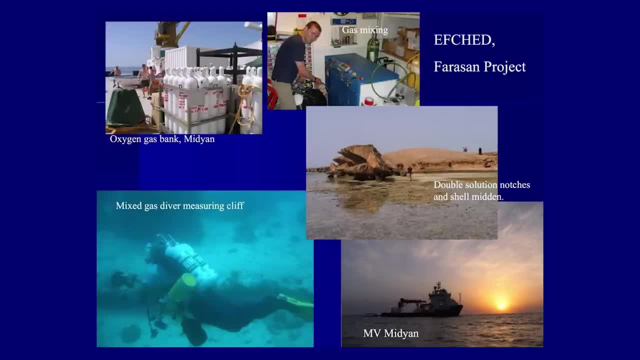 Various scenes during the Farasan Island projects. Divers have been going out there now almost every year for five or six years and last year, 2013,, we had the Greek research ship with Dimitris Sakalarou, their ship Egeo, taking soundings in those deep wells, deep pits. 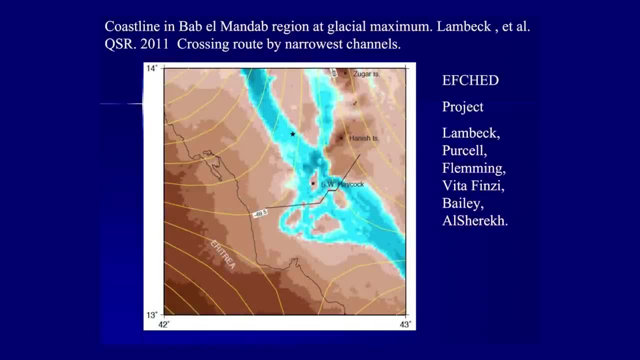 This is a reconstruction of the most likely crossing point. The Hanisha Islands are here. The shallowest point is there, but it's not narrow. It's about 10 kilometres. Once water is too deep to walk in, it's the width which determines. 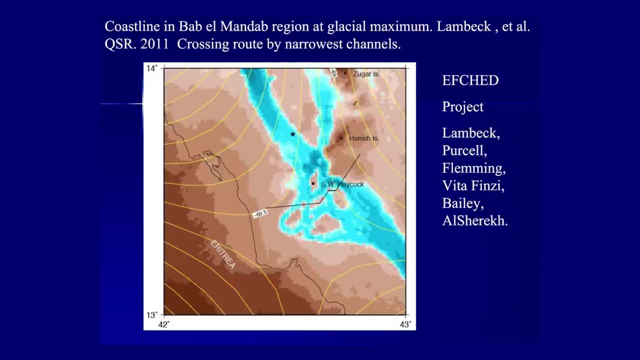 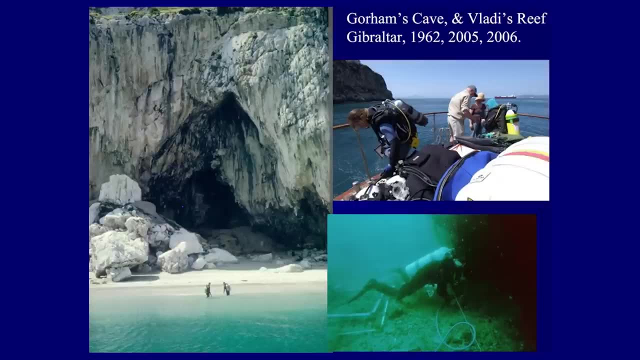 whether people cross it and that's the most likely crossing point: Gibraltar. a whole lot of caves there and Clive Finlay said and others Darren Farr, have been working there for years, also with Chris Stringer reconstructing the occupation. 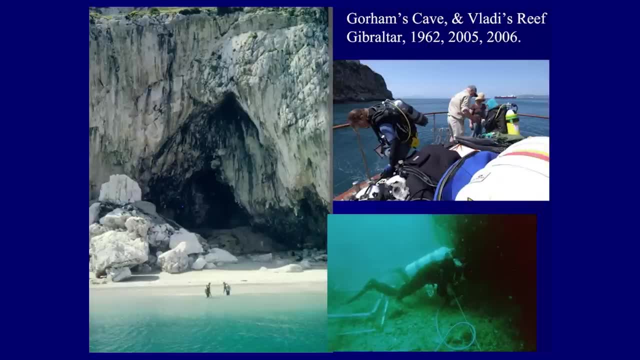 of these caves. I found caves here in the 1960s and since then we've been surveying them and worked out that this reef is about 30,000 years, or older than 30,000 years, with caves in it, and probably has Neanderthal remains. 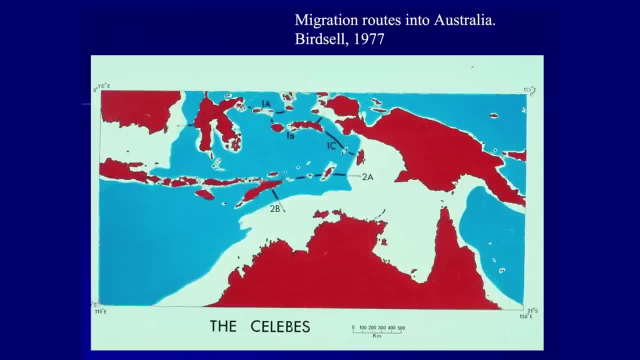 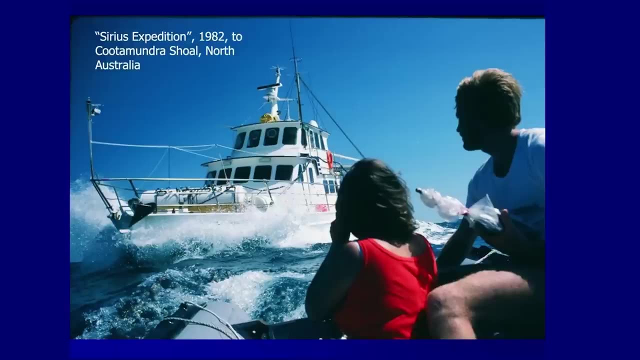 Australia in the 1980s I went out there with Jay and in fact also our daughter was four months old at the time. quite adventurous, She's in that ship. I don't think Kirsten is here. Anyway, the recompression chamber: divers working here. 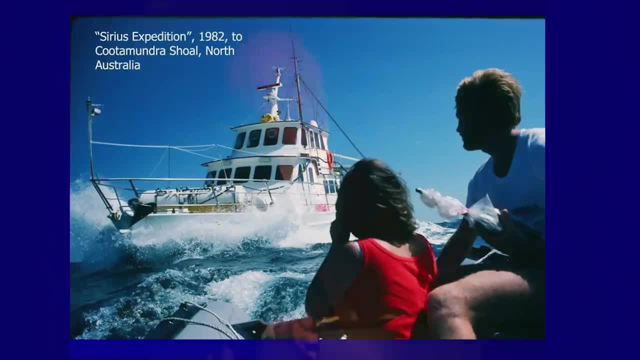 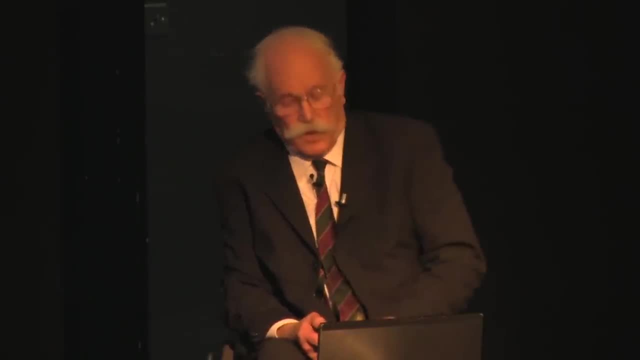 The reefs are about 32 metres- 36 metres down, so there's very little shallow diving. The Kutamandra Shoal comes up to 15 metres at one place, but most of the diving was in 30 to 60 metres. 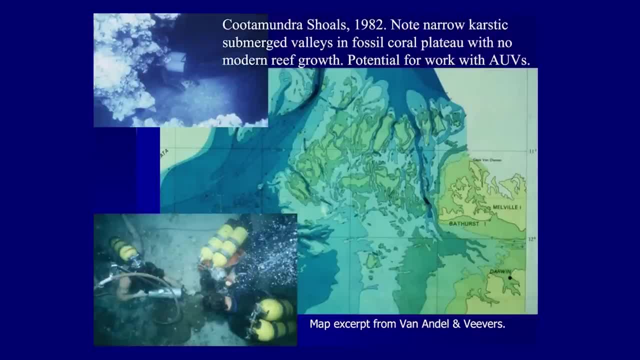 We're about 200 metres down, We're 200 kilometres out from Darwin, and that's the place where we were doing most of the diving, and in those valleys It would have been perfect sheltered conditions, protected from storms, and there would have been mangrove forests. 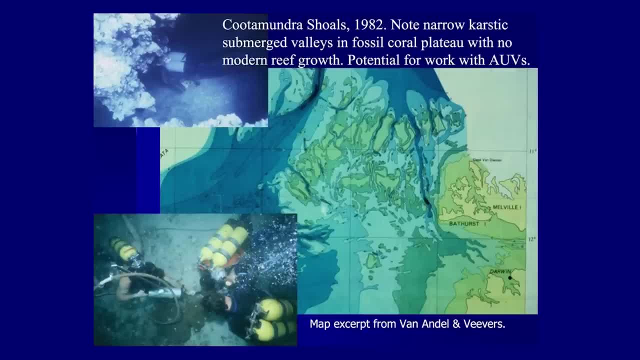 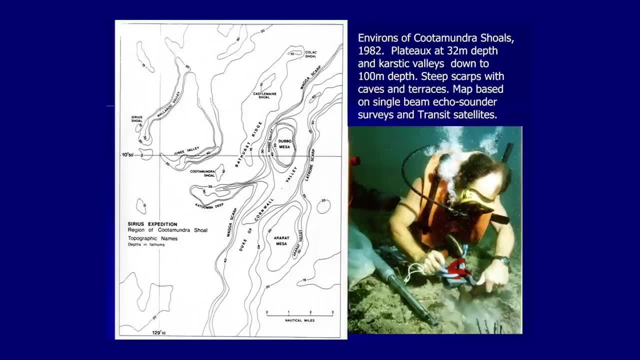 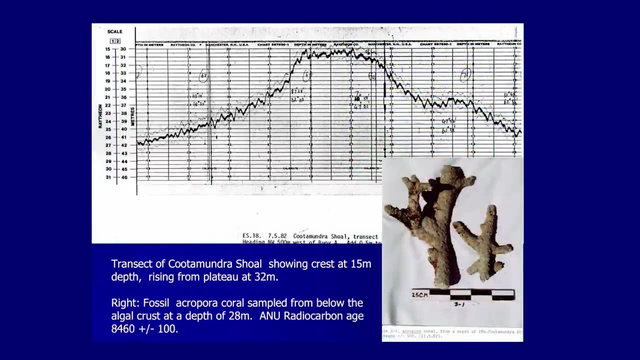 and plenty of good food for the Aborigine peoples moving into Australia. One of the maps that we made of the terrain in 1982, Karl Shaw working at 40 or 50 metres with a rock drill Cross-section of the reef itself: Kutamandra Shoals. 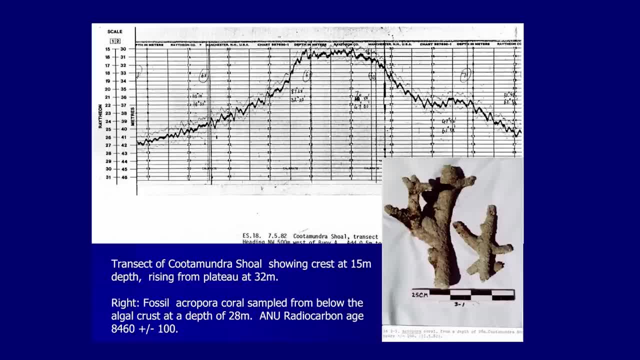 and we took a number of coral samples. There's no modern live coral, which means that the sea floor is, in effect, the Ice Age terrestrial landscape, which was the reason why I wanted to work there. You break through the crust on the surface. 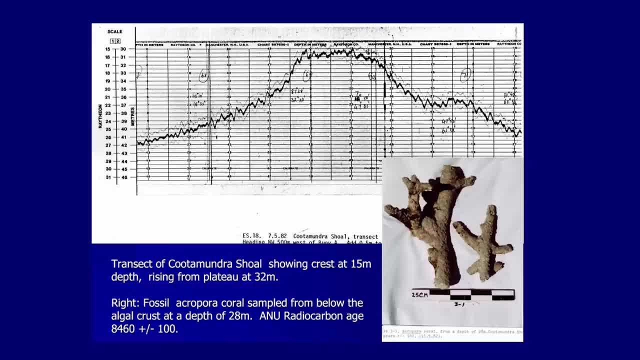 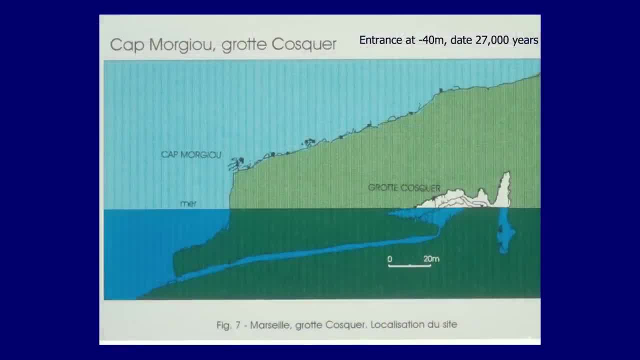 and there is coral underneath of older sea-level periods when the sea was coming up South of France. I did a lot of diving here in the 1960s, but unfortunately I did not find this cave which was discovered by Georges Cosquer. 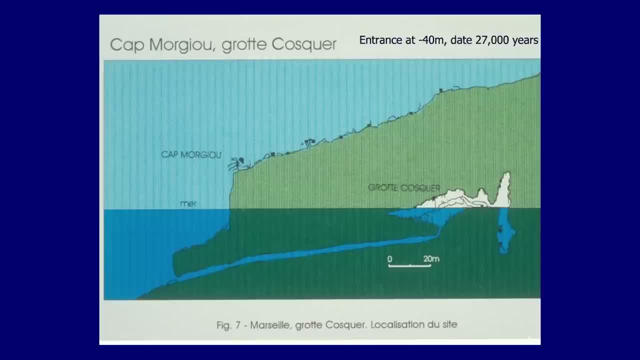 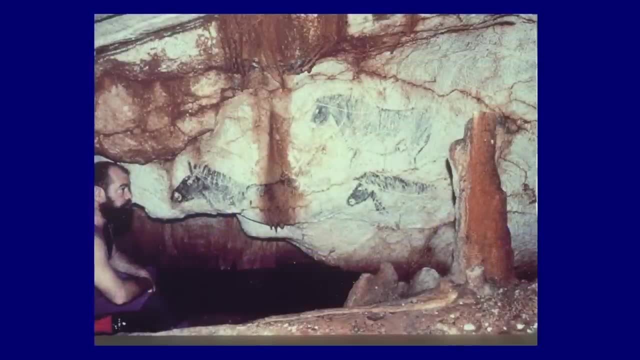 sorry Henri Cosquer- in the early 90s and when he swam up that tunnel. this is what they found inside. For a while the French authorities didn't believe it and thought that the divers had painted these things as a joke. 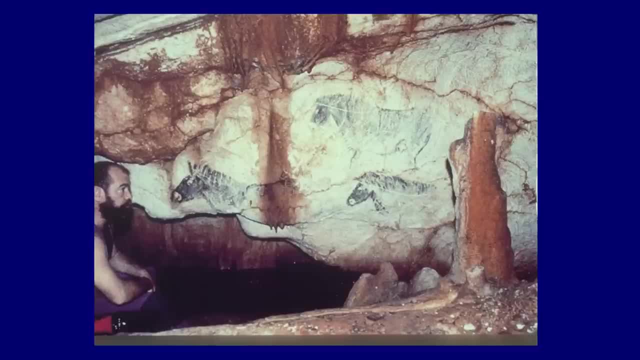 but they- Not many divers, not many professional archaeologists were prepared to go down 40 metres and swim up that tunnel. but it is absolutely genuine. I can assure you I love this reconstruction. There's a magnificent book by Clotes and Cortin. 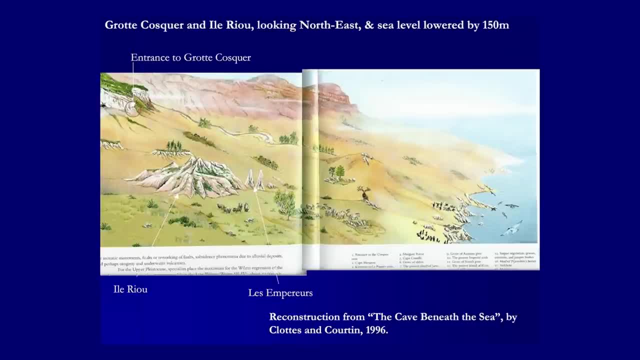 There's the entrance to the cave. I dived all around these islands, including 80 metres down one of those pinnacles. It's a lovely attempt- and very unusual, to try and reconstruct a visual impression of what the landscape was like at this time. 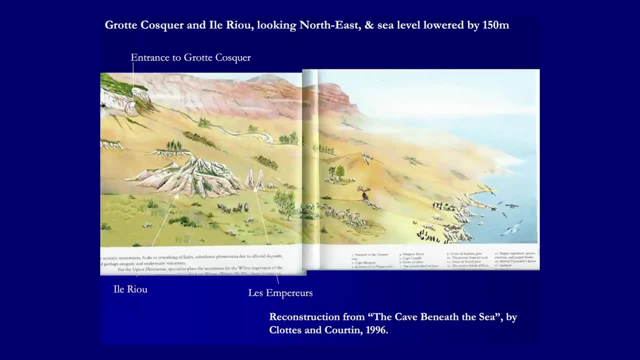 but if you look at the scale, that's about 100 metres. Here we have a sort of elk and the humans are about 10 or 20 metres high. but still, all credit for trying to show what the continental shelf really looked like. 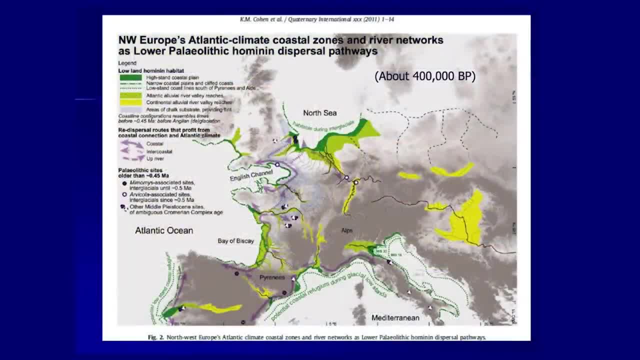 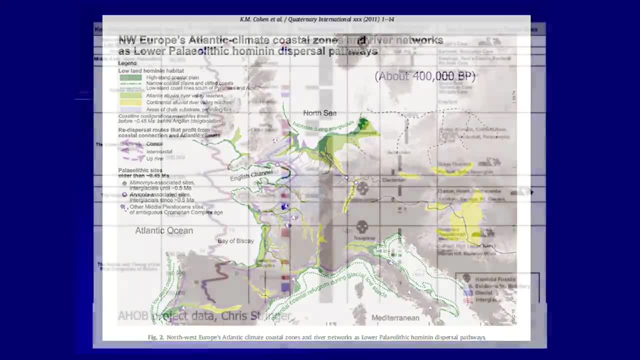 Back to the North Sea. we're going back now 100,000 years or more. The Weald Artois Ridge joins Britain to the mainland and this is from Chris Stringer's AHOB project. Britain was joined to the mainland. 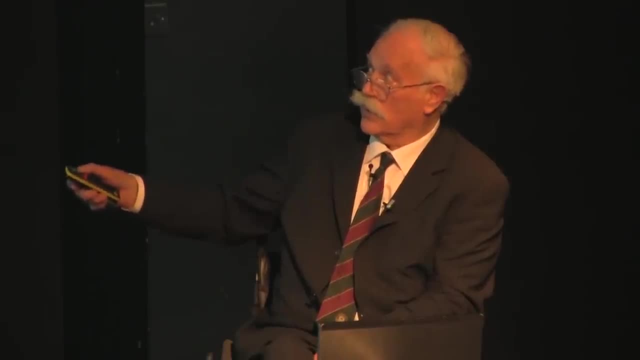 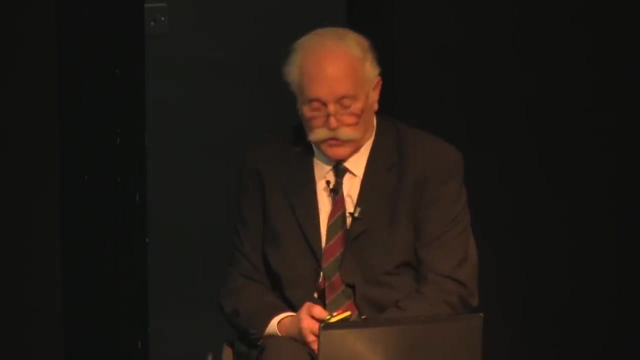 and there's a solid bar there and was an island only at those occasions. So most of the last 650,000 years we've been joined onto the mainland of Europe. Mammoth and other bits and pieces come out of the North Sea all the time. 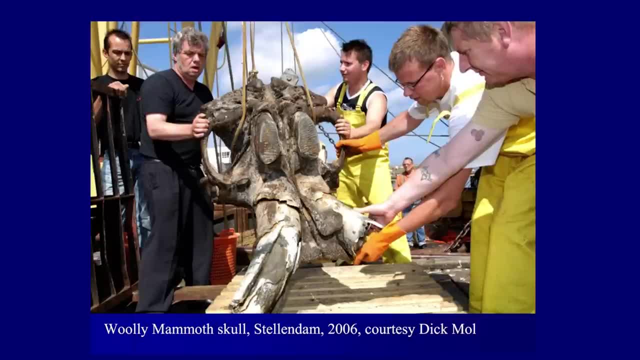 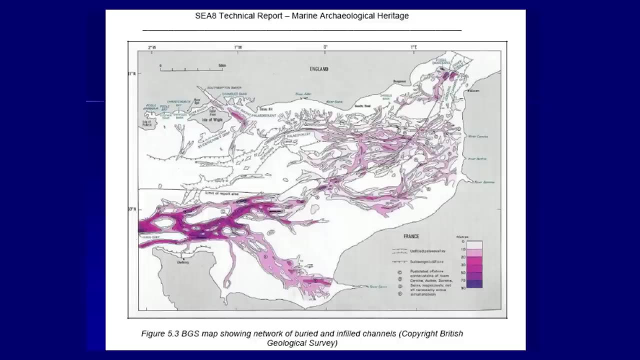 This skull is in the offices of Klaas Post in Urk, and many other pieces like that have been found year after year by the fishermen. The English Channel- This map shows the Weald Artois Ridge has gone, but you've got all the river valleys. 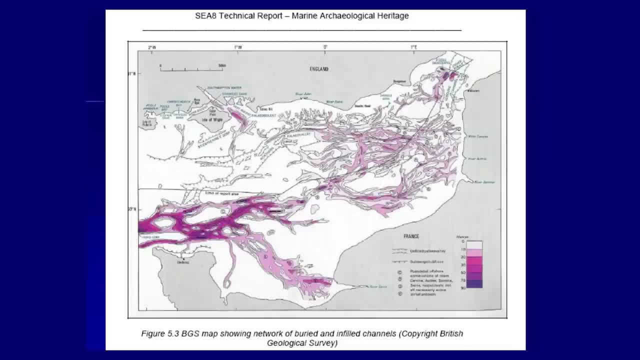 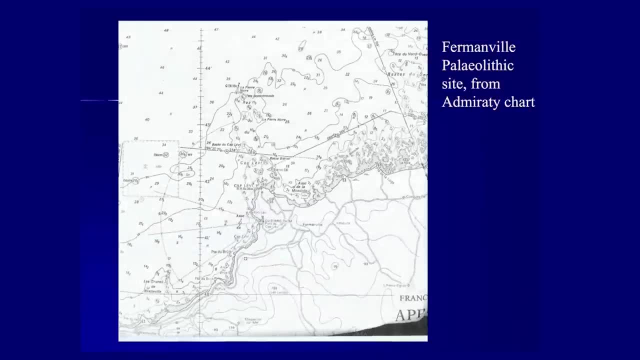 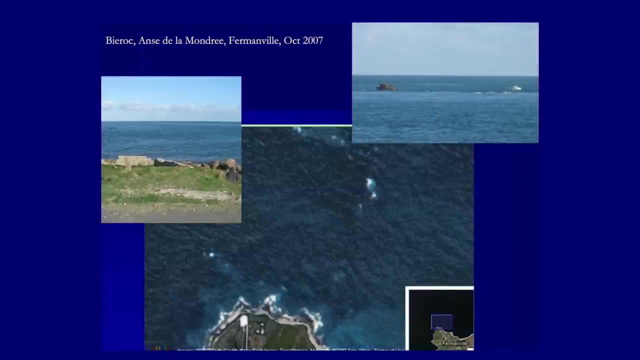 coming down into what's called the Channel River, which goes just past Cherbourg. here, Cap Lévis, near Fermontville on the chart is a granite ridge going out like that about a kilometre or more. On Google Earth you can see it here. 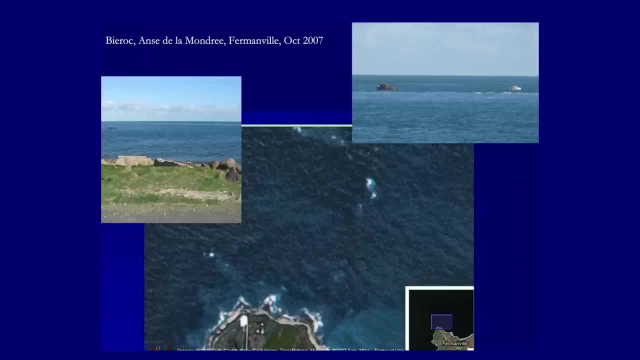 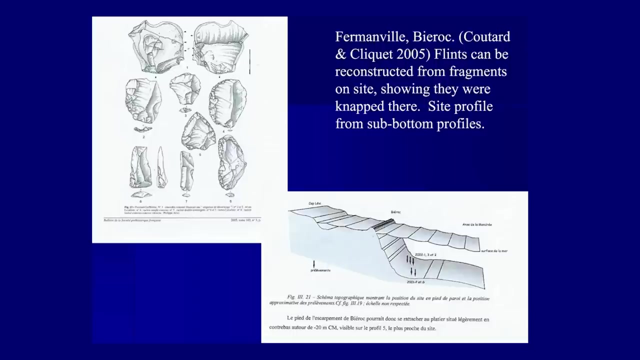 This little rock's called the Biais Rock. Jay and I went out there in 2007, and you can see the current flowing over that reef When you dive down there. there are stone tools everywhere. This was actually found and first documented. 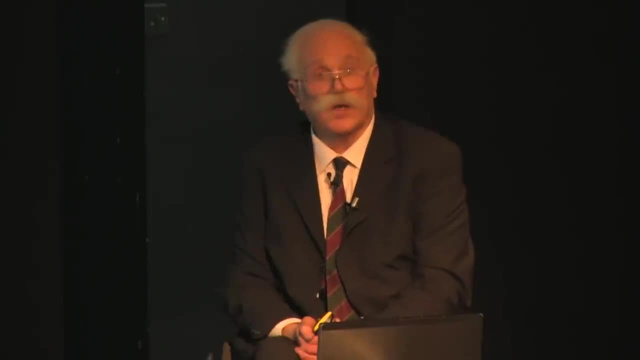 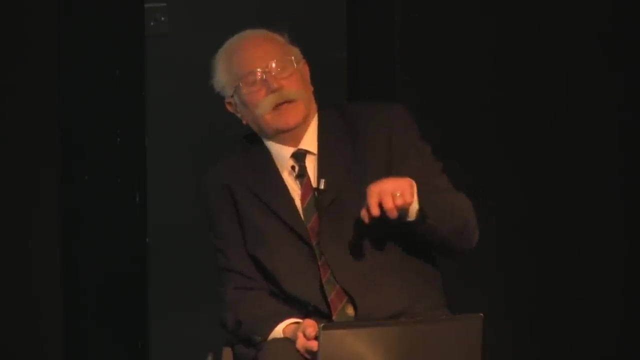 by Scouvet and Verag in 1978, a really revolutionary document. Hardly anybody's read it. If you look it up on the web, it always cites me as having cited Scouvet and Verag, But I can assure you. 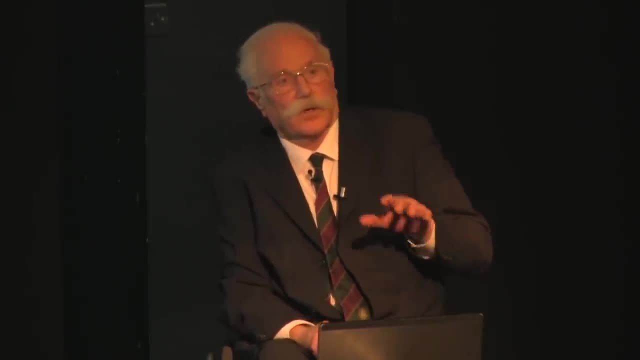 if you can get hold of the original. it's an astonishing piece of work. They studied the solid geology, earth movements, climate change, sea level change, sediment movement, the archaeology, the preservation of the artefacts and so on. 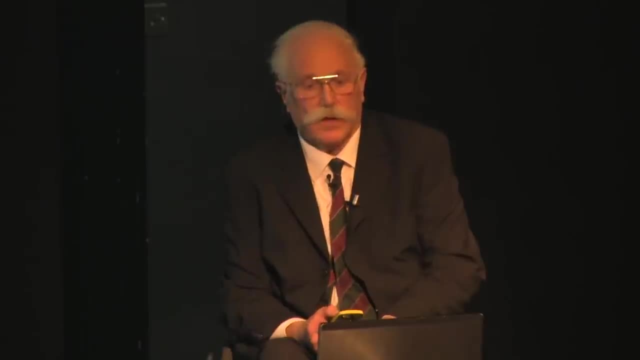 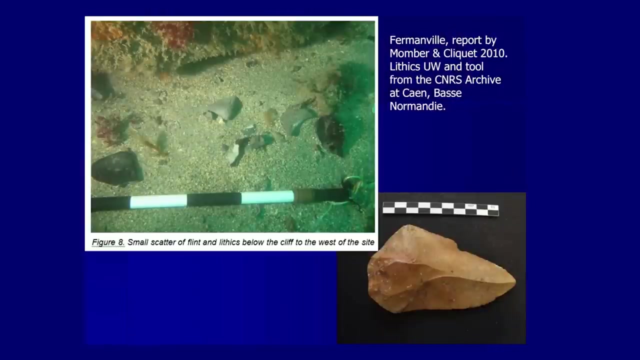 in a volume of about 150, 200 pages, And there are very few projects like that. We've been going back there now to try and reinterpret it with modern instrumentation and modern analytic techniques, And I've been working with the French Oceanographic Laboratory at Ifremer. 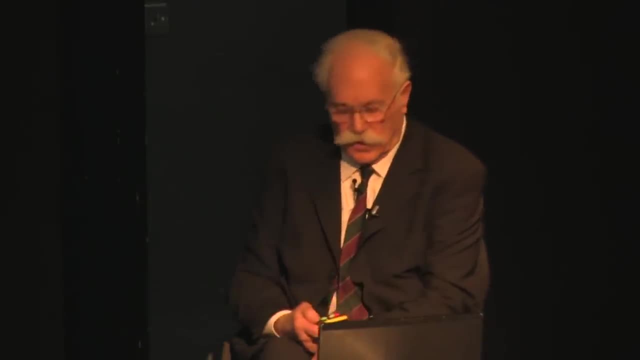 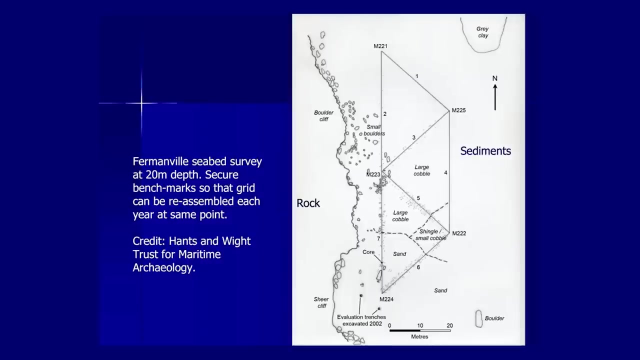 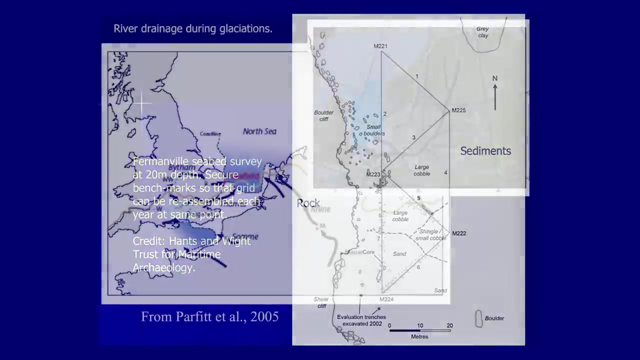 to try and arrange so that we can do some really accurate sonar mapping of the site. That was the map which the French and British divers made a couple of years ago. I don't have the date there. Okay, now we're getting back to really old sites. 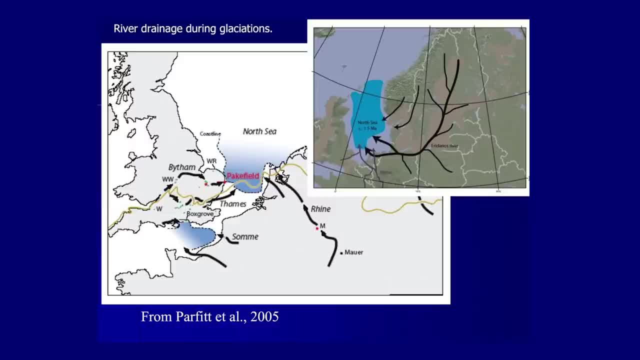 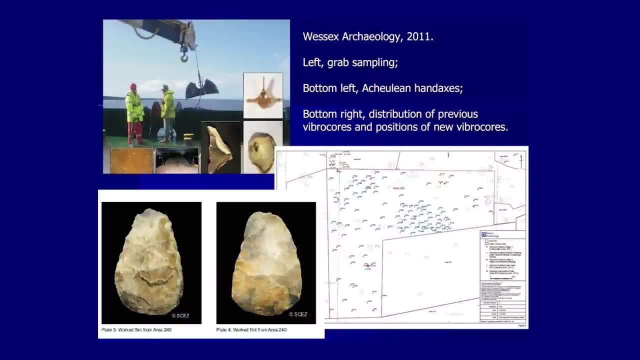 The Weald Artois Ridge is now in place. We're in the North Sea and the very old British sites are here: Stone tools, Acheulean hand axes, 70,000 years old. And then, when the site was investigated, 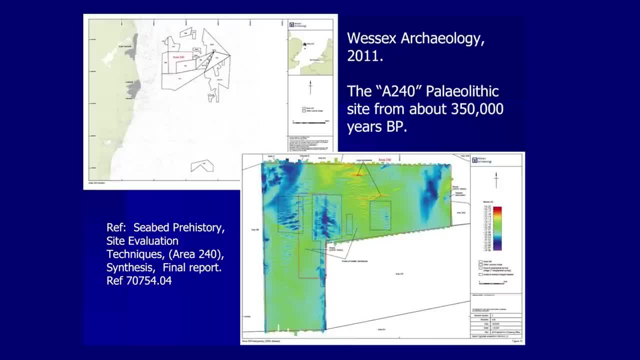 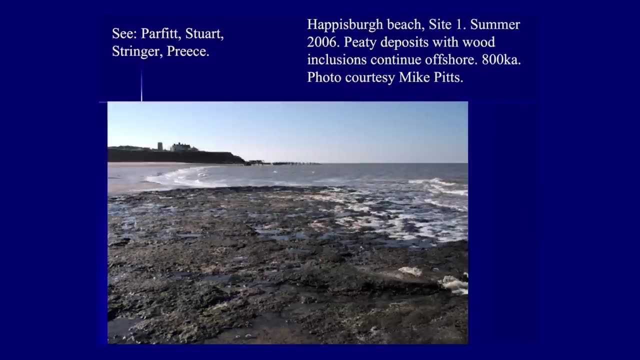 by Wessex Archaeology. with coring through the sediments they got down to layers where there were tools or flakes of work flint in sediment layers 350,000 years old. in the centre of the North Sea, On the shoreline we have material which is 800,000 years old. 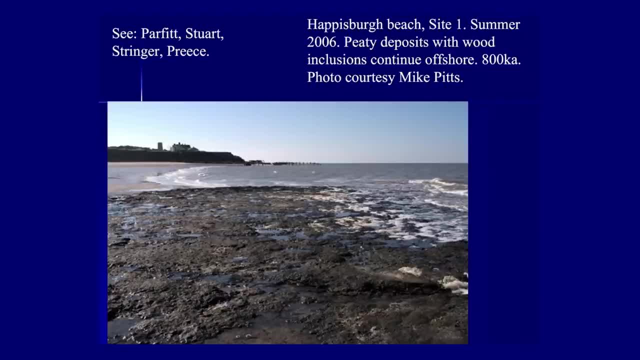 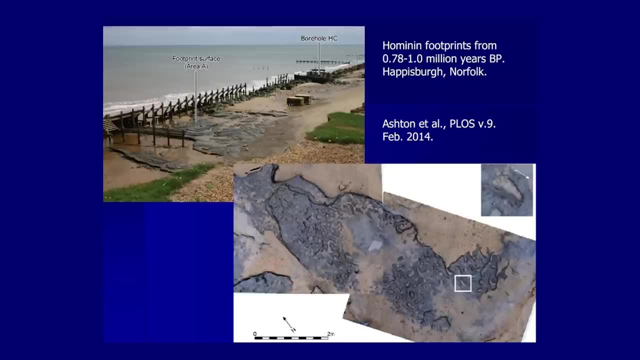 quite close by And you probably saw in the popular press last year, footprints found in fossil mud- And that's from the paper- 0.78 to 1 million years old, And they were washed away and destroyed by the storms which came up last winter. 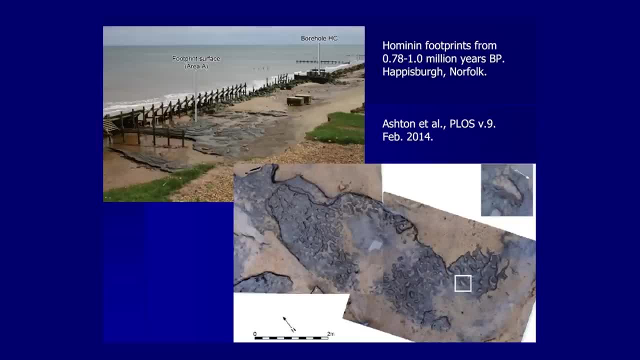 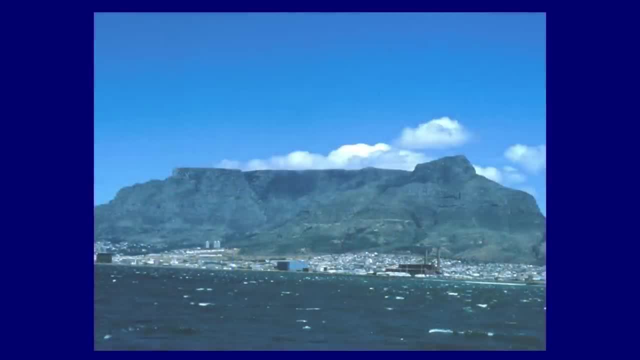 But that data has been published showing the footprints of a family walking along the beach at least 800,000 years ago. Cape Town. I went out there in 1995 to give a lecture And as I was preparing my talk, Bruno Wirtz came up to me. 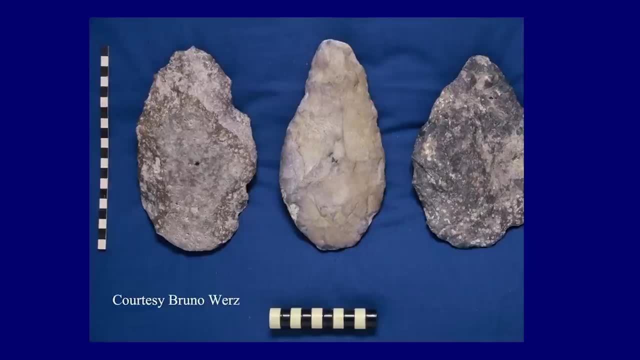 and showed me these hand axes which some divers working on a Dutch East India wreck had found by mistake, And nobody locally realised how important it was. I was absolutely astonished and worked with Bruno to get that published. Nature didn't like it, so we published it in the Journal of South African Science. 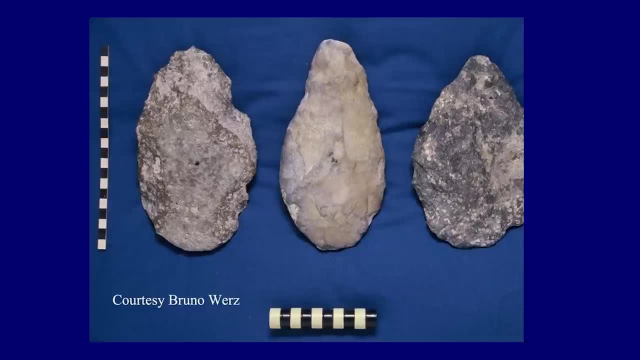 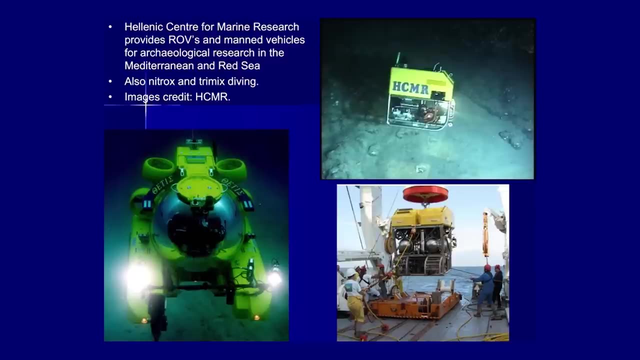 And they are the oldest human artefacts ever found under the sea. To look at the technology that we've been using, I've mentioned diving and sophisticated gas mixtures, autonomous underwater vehicles. The Greek Centre for Maritime Research is using both manned vehicles and robotic vehicles. 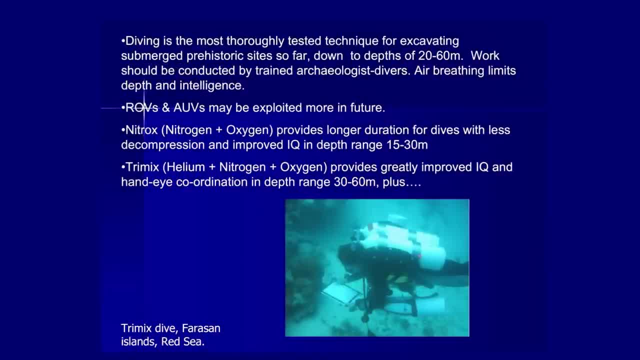 Gas mixtures when diving are very important. There's no point in taking a PhD diver making them breathe air so that their backs are 2A levels at 20 metres, O level at 40 metres and kindergarten at 50 metres. 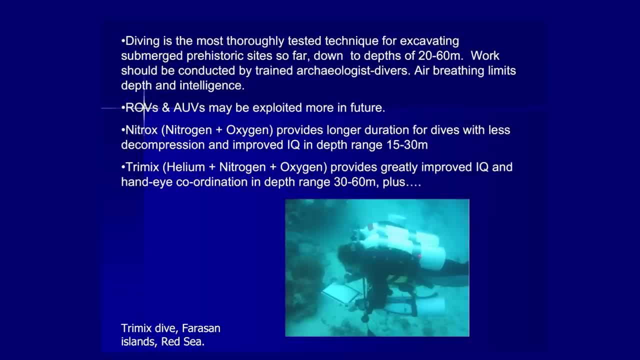 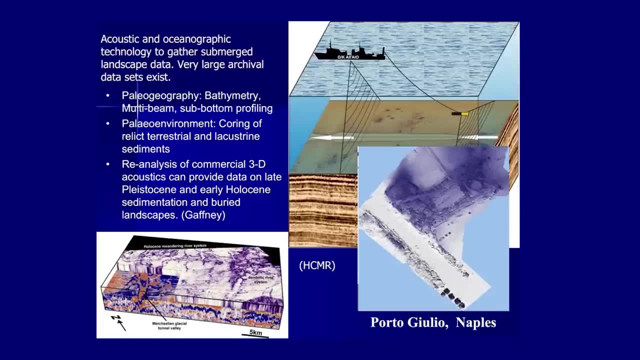 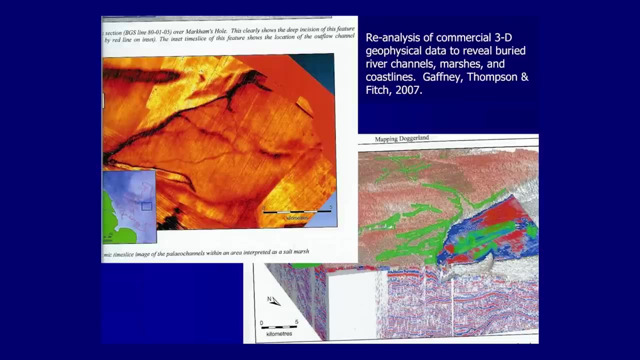 So give them a good gas mixture so that they preserve their IQ. Acoustic methods: astonishing techniques are now available for mapping inside the sediments and to reconstruct incredibly accurate topographies of marshes, swamps, shorelines, caves and so on. 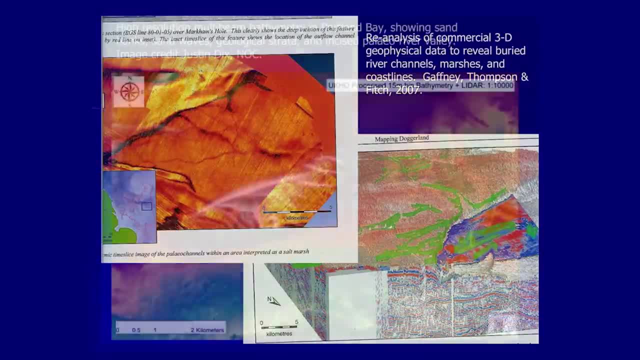 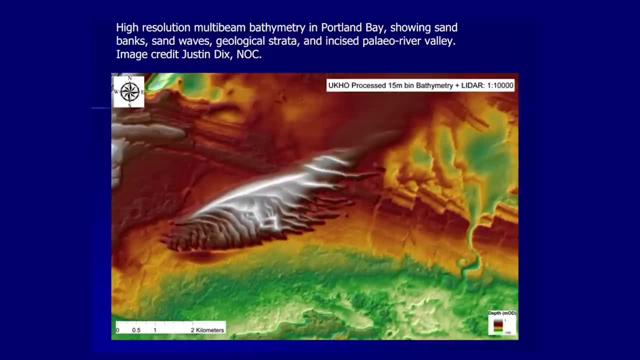 both within the sediments and on exposed bits of the sea floor. This is a fabulous reconstruction of The Portland bill is just here, Rocky Headland. The eddies which go round here, that's two kilometres, form this fabulous, huge. 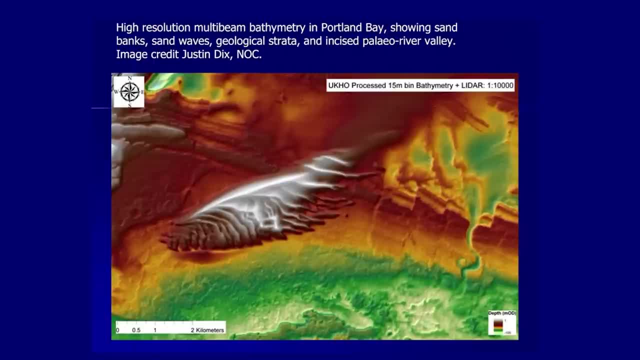 sort of dynamic sand dune which looks almost alive. You can see the sand waves and currents are rippling off it. Underneath the mobile sediments you've got the bedrock. you can see the dipping plains of rock. you can see the faults in the bedrock. 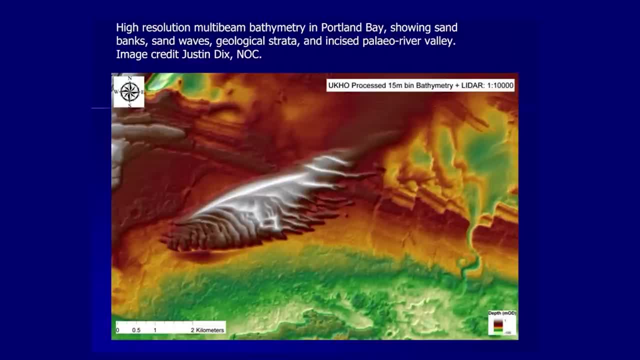 and even there a river valley going through the rock and incised meander. You've probably got half a million years of climate and geology in that one image, all done by acoustics. That would have been absolutely impossible 20 years ago. 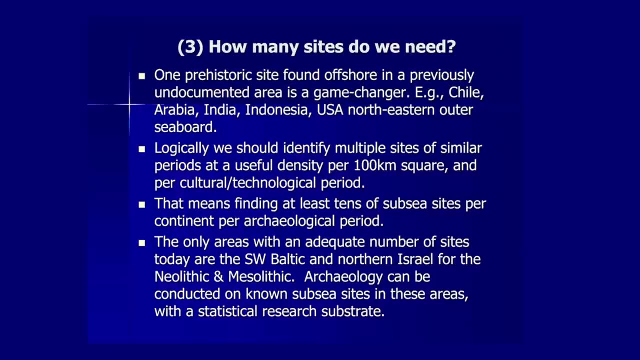 OK, I asked how many sites would be needed. Ideally you want tens of sites in a 100-kilometre square. There are whole continents where we've got one or none. The entire southern route from the Southern Red Sea round India, Southeast Asia and Indonesia. 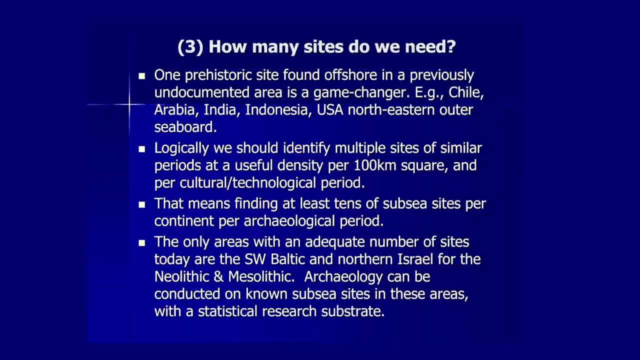 there are no known submerged prehistoric sites And yet it's obviously staggering and important both for human diffusion through the Asiatic continent and for the occupation of Australia. We are finding them, but the only area where you can do what I call modern archaeology. 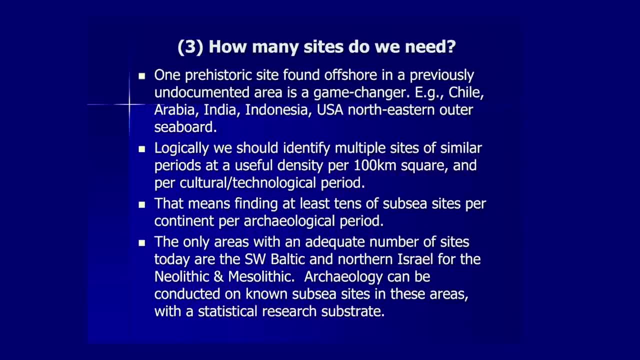 studying dozens of sites. thousands of artefacts and changes spatially and in time are in the Southern Baltic parts of the North Sea and the coast of Israel. So there's an enormous amount of work to do. If we look at the numbers of sites in Europe, 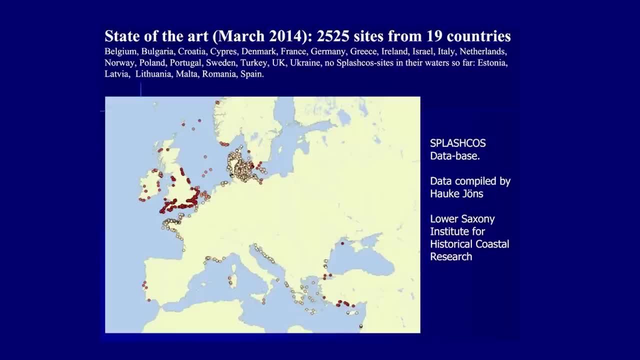 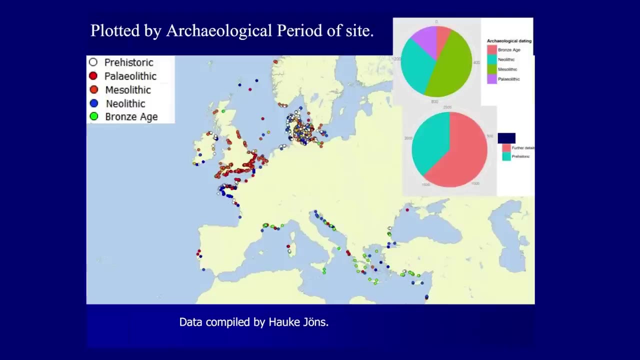 this is from the SPLASHCOS database. You can look these things up on the transcript. There's over 2,500 sites and some missing. Not all countries have returned their data. We can look at them distributed by age. As I say, when the data came in. 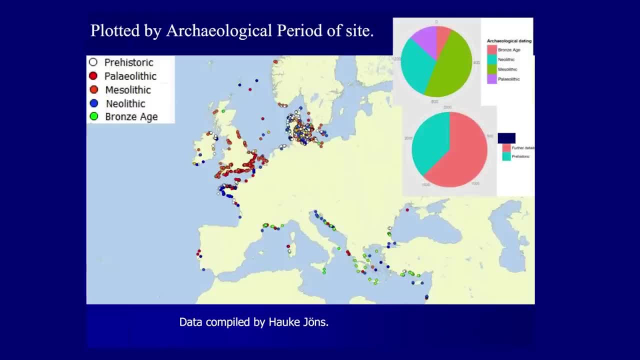 I was quite astonished how many were in the late Paleolithic. And also you can see that material survives in very widely different environments. The Yugoslavian coast is sort of rocky and steep with dozens of islands. The Baltic is all sediments and mud and low islands. 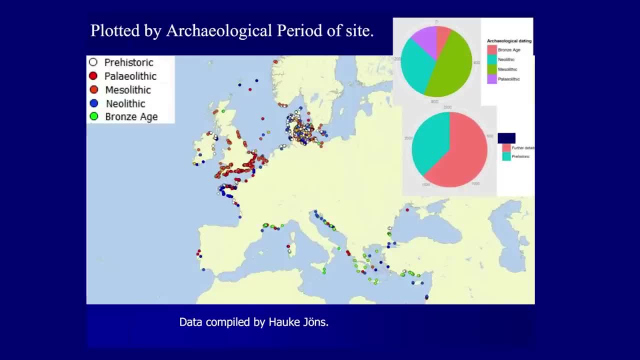 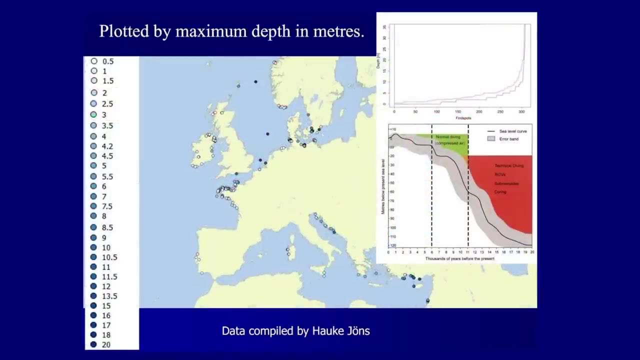 The coast of Israel is straight sandy beach, with 1,000 kilometers of fetch, of waves breaking on it and so on, So sites can survive in all sorts of different geomorphological environments. The map on the right showing, or the diagram on the right showing, the diving depth. is a little bit conservative. for air diving You can probably work down to 20 meters quite well on air, But nitrox around 20 to 30 meters to reduce nitrogen narcosis and then trimix down to 80 or 90 meters. 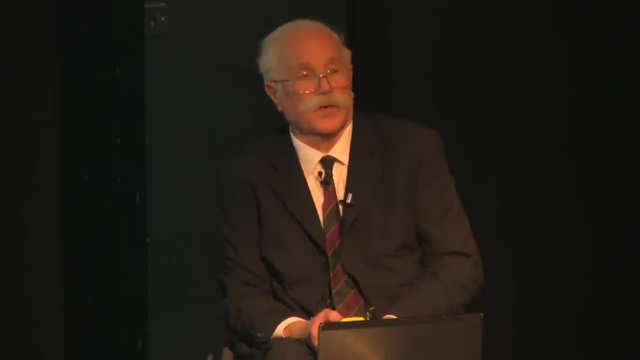 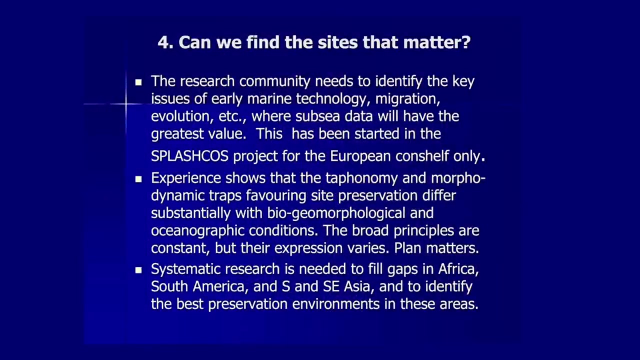 Up to this point, no prehistoric site has been excavated or studied in detail by any means other than by diving, although we're obviously working on robotic techniques Finding the sites that matter. Again, we're putting together a strategy. We're getting there. 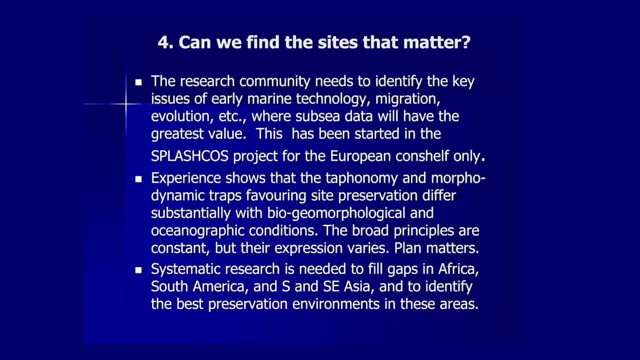 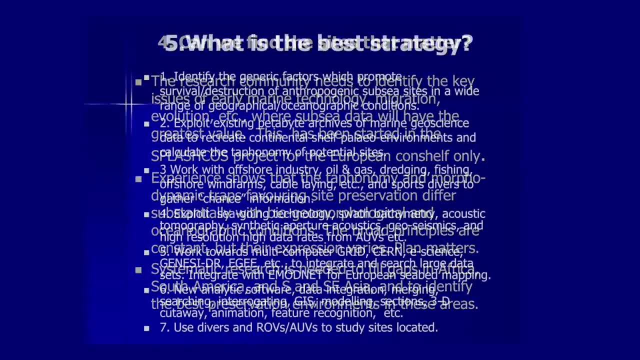 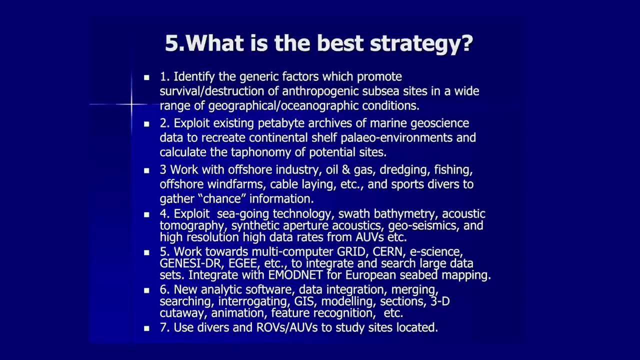 The systematic research strategy is only just being developed at a continental and global scale, but we are working on it. Don't try and read all the small print. This is an outline of the strategic methods that we're developing for European programs funded through the Commission. 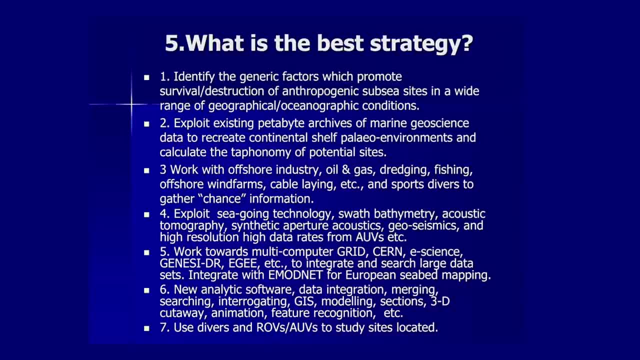 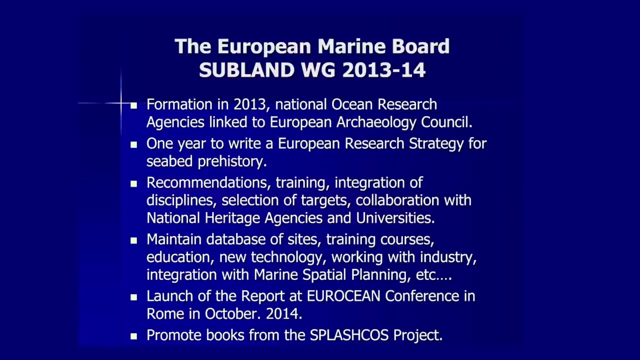 to study different aspects of prehistoric archaeology around in the European seas, And I'm now chairing a working group known as SUBLAND, which is sponsored by the European Marine Board, has representatives from about 15 different countries and is working with the European Archaeology Council. 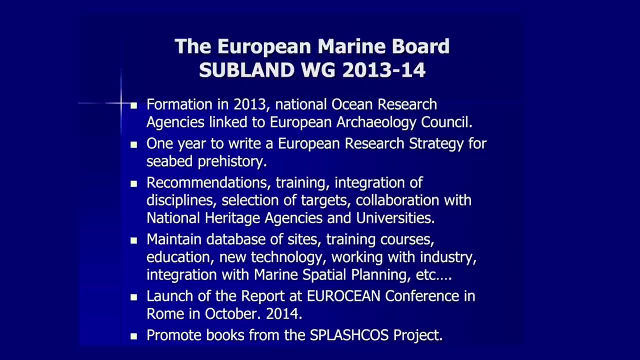 to develop a multidisciplinary research strategy looking ahead five or ten years. We have no authority to actually decide policy or instruct anybody to do anything, but I hope that the combination of skills that we're bringing together, the range of experience, the results of surveying national policies, 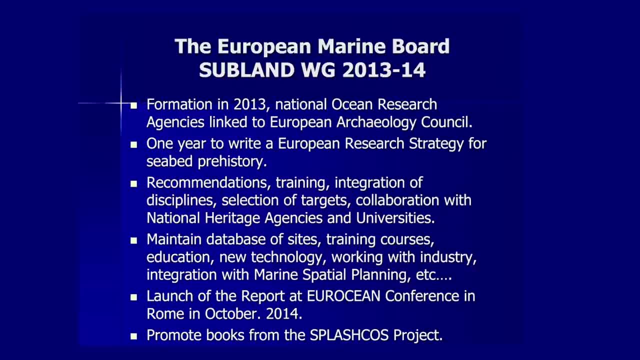 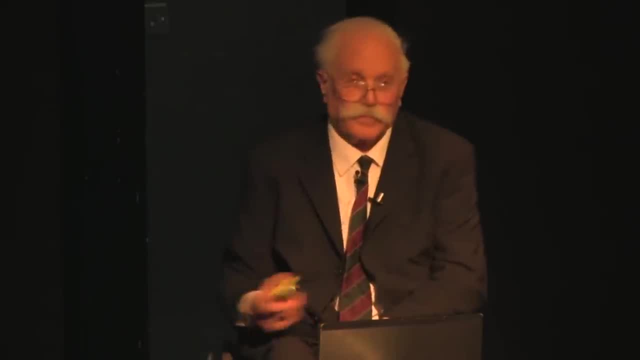 for submarine prehistoric research through the National Heritage Agencies, plus all the technology and skills from the oceanographic laboratories of the Marine Board, we can show that the strategy we're putting forward is sensible. Thank you very much. Thank you very much.